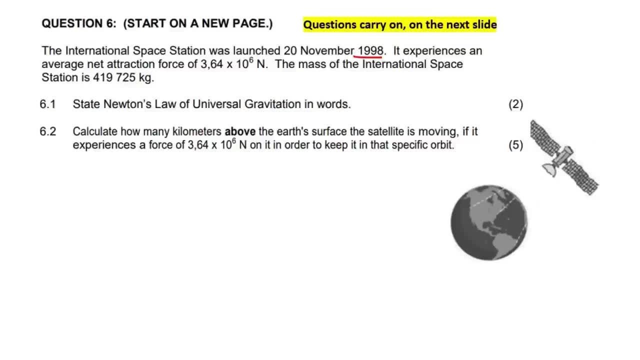 at that, 419,000 kilograms. This is a big object. So some of you like super nerdy people out there are like yo, dude, it's the space station, Don't you know like, and to be honest, I don't like I. 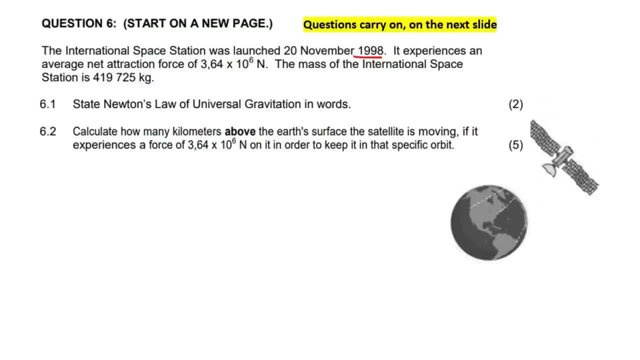 don't actually know a lot of these things. It just doesn't fascinate Me. But I know some people love it. They like have like pictures of all the stuff on their wall and stuff. But that's awesome. It's like future Elon Musk in the house. So 419725 kilograms- Okay. 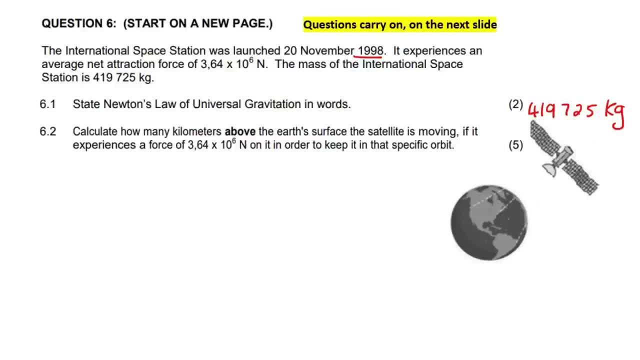 so the first question says: state Newton's law of gravitation and words. Now, let's first, before we go, get our form and our definitions, Let's think about the formula of Newton's law of gravity. It goes like this, And so check this out: The net force acting on the force of gravity is the force. 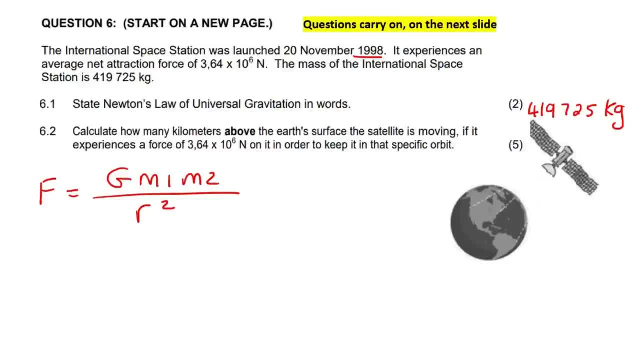 of attraction between two objects is directly proportional. directly proportional means all the things that are in the top to the product. These means product of the mass of the objects and, indirectly, which is at the bottom proportional to the. there should actually be a D proportional. 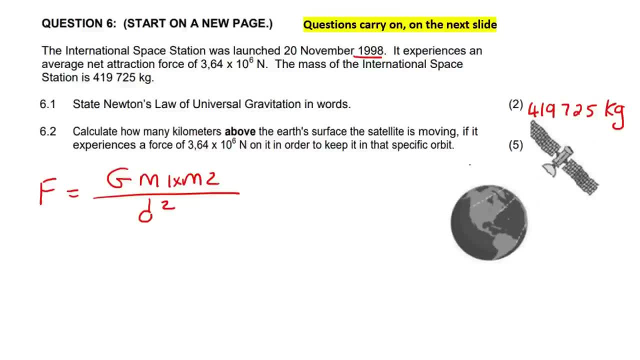 because sometimes it's an R, sometimes it's a D, depending on whether we have an object that's on the surface, because then the distance between them is the radius. Okay, but it's actually correct to rather use a D, because sometimes the objects not on the surface, And so you're measuring that distance there, Okay. 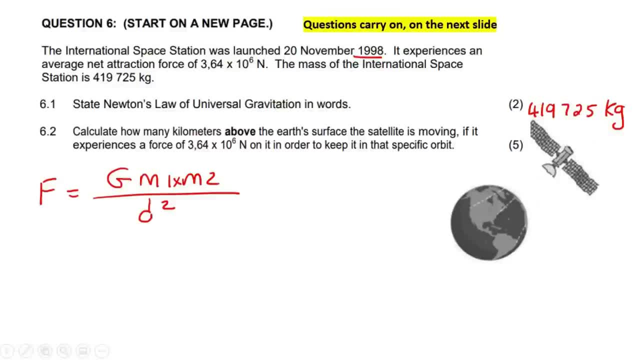 so it's not the radius anymore. Sometimes I use it interchangeably. they don't mark you wrong in the exam, So okay. so we said directly proportional to the product of the mass and inversely proportional to the square of the distance between their centers. Now let's go right to. we'll find out. 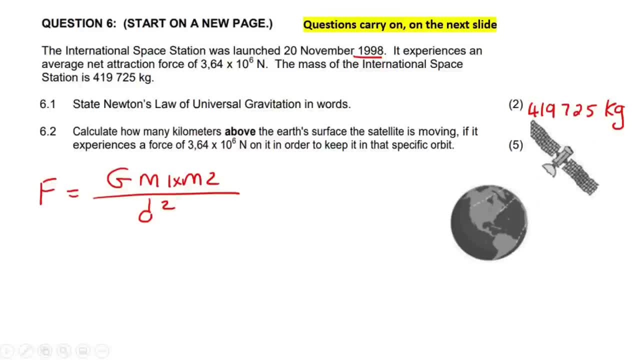 the formal definition, But what I like to do is always look at the formula, because it gives me a reminder when I'm sitting in my exam And I'm anxious as anything of what the definition tells me. and then a triggers all of those little synapses. 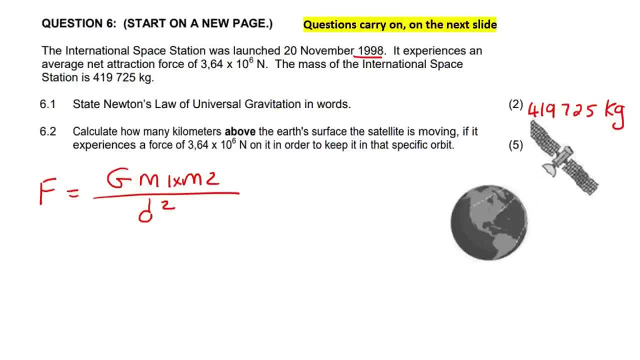 in my brain: Okay, why are you getting so technical, bro? Why are you flexing that? you did Life Sciences like 10 years ago back in high school. Sorry, guys, I just had my moment there. My mom would be proud, Okay. So, yeah, I like to. I like to keep me so fancy saying synapses. I know guys. So 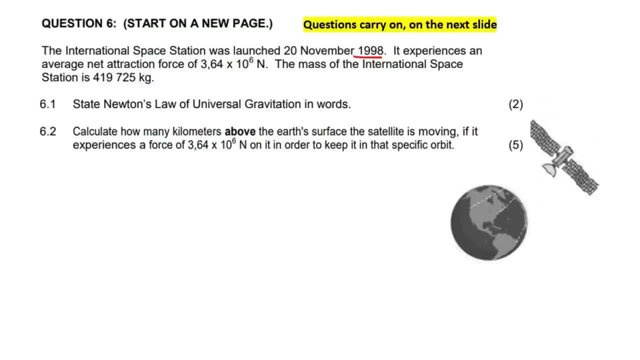 don't actually know a lot of these things. It just doesn't fascinate me. But I know some people love it. They like have like pictures of all the stuff on their wall and stuff. But that's awesome. It's like future Elon Musk in the house. So 419725 kilograms- Okay. 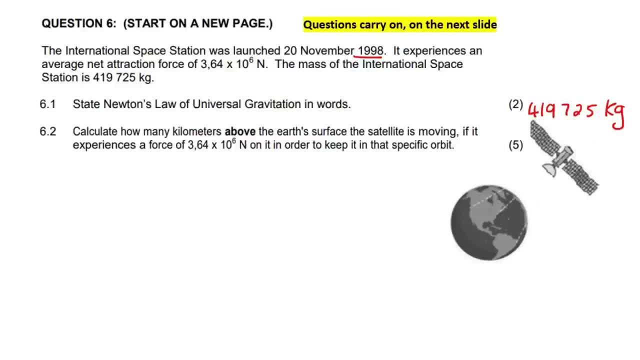 so the first question says: state Newton's law of gravitation and words. Now, let's first, before we go, get our form and our definitions, Let's think about the formula of Newton's law of gravity. It goes like this, And so check this out: The net force acting on the force of gravity is the force. 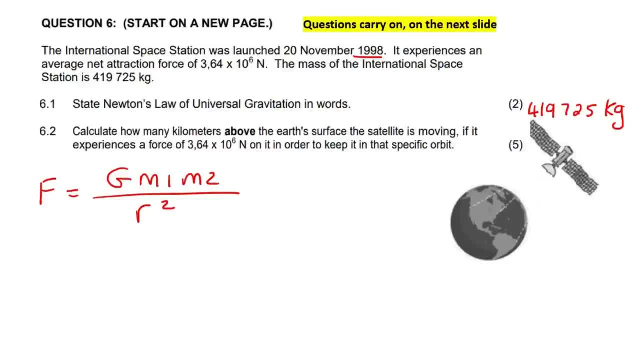 of attraction between two objects is directly proportional. directly proportional means all the things that are in the top to the product. These means product of the mass of the objects and, indirectly, which is at the bottom proportional to the. there should actually be a D proportional. 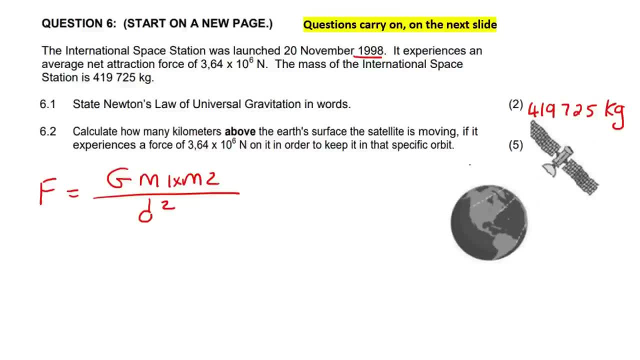 because sometimes it's an R, sometimes it's a D, depending on whether we have an object that's on the surface, because then the distance between them is the radius. Okay, but it's actually correct to rather use a D, because sometimes the objects not on the surface, And so you're measuring that distance there, Okay. 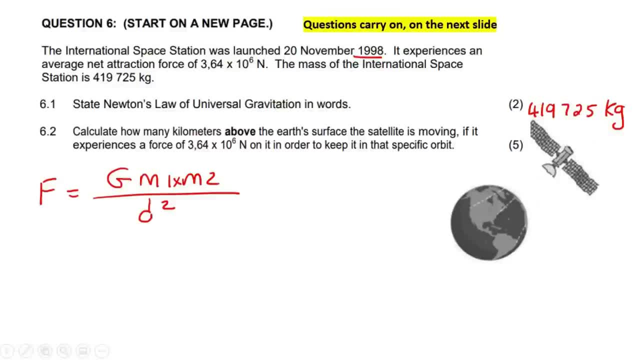 so it's not the radius anymore. Sometimes I use it interchangeably. they don't mark you wrong in the exam, So okay. so we said directly proportional to the product of the mass and inversely proportional to the square of the distance between their centers. Now let's go right to. we'll find out. 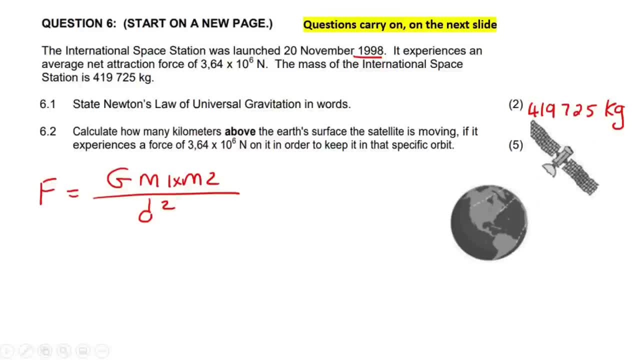 the formal definition, But what I like to do is always look at the formula, because it gives me a reminder when I'm sitting in my exam And I'm anxious as anything, of what the definition tells me. and then it triggers all of those little synapses. 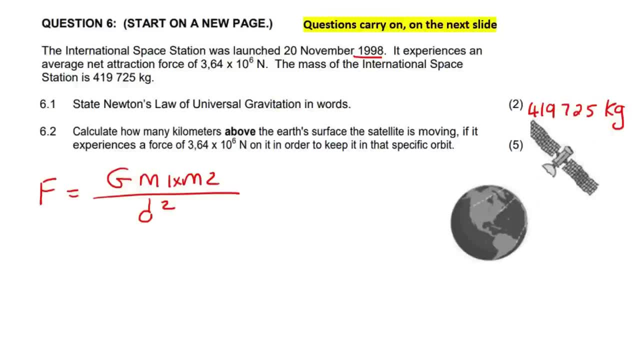 in my brain: Okay, why are you getting so technical, bro? Why flexing that? you did life sciences like 10 years ago back in high school. Sorry, guys, I just had my moment there. My mom would be proud, Okay. So yeah, I like to. I like to Kevin, you so fancy saying synapses. I know guys, So so you take. 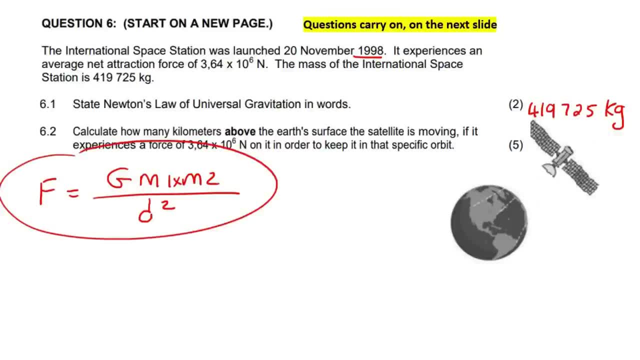 so you take this formula and it helps to trigger the definition. okay, so let's go get the definition now. and so here it is, guys. so every particle in the universe exerts. now, this part might be different to what your teacher says, but you see that they're not actually marking you on that first part. the underlined part is where 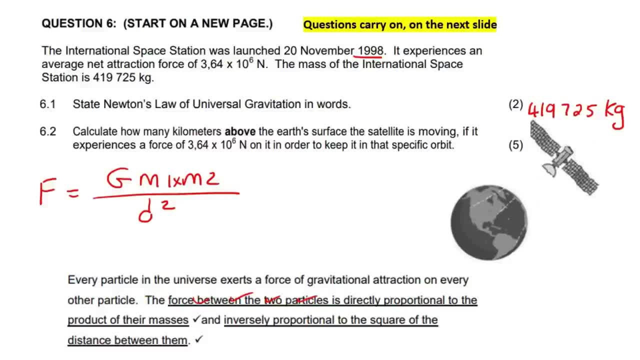 they really care. the force between the two particles is directly proportional to the product of their mass and inversely proportional to the square of the distance between them. usually this is between their centers, but you see, it changes. it's not exact. okay, so if you said between their centers, then it's fine. it's only when you are in a specific high school where your 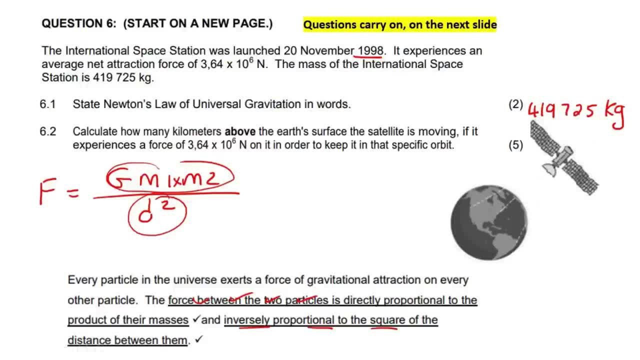 teacher thinks that they are the godfather of definitions and their method and their wording is the only way. but that's just silly, um, come on, come on. we live in a big world where everyone's got. you know, different schools have different, different, different definitions, and so here we. have like an official exam paper where everyone gets the same definition of setting a learning plan in two days. every class has a different. any campus has another ongoing class. didn't edit it. every class has a class and so on and so on. in right schools get different patterns, for those grow advantage. 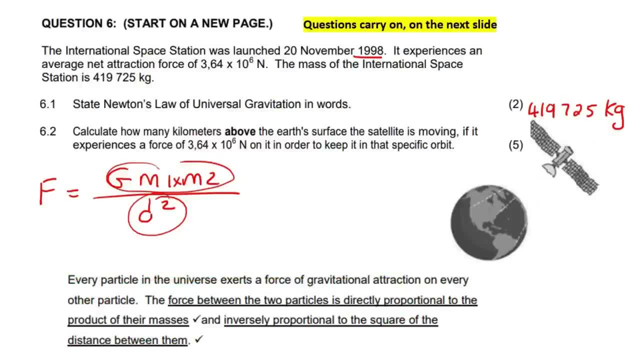 Where you see they're not looking at the first part And your teacher might be like you need to get that every single part. And don't you dare leave out the word, the Don't you dare. And don't, oh, don't you leave out that. 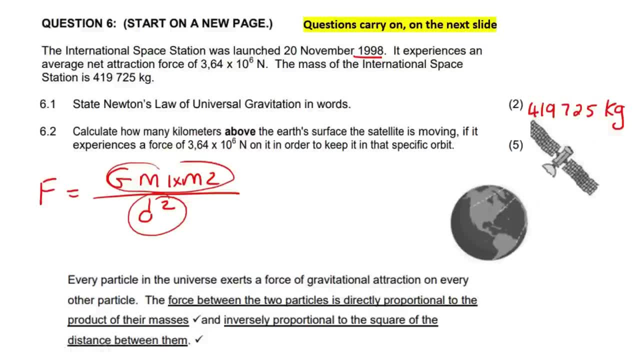 I think it's so silly, to be honest. But anyways, what can we do? So we can protest, Kevin? Okay, Let's not start a rebellion here. Okay, So I'm a silly man, aren't I? 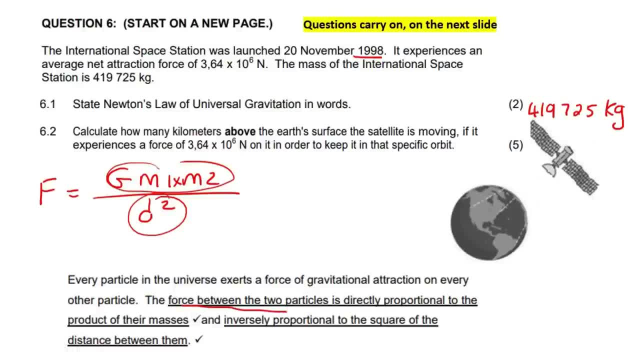 Okay, So then we just these are the important parts that they're looking for. Okay, I didn't underline this, by the way, This is literally from the memo. They underline that, So that's what they're looking for. 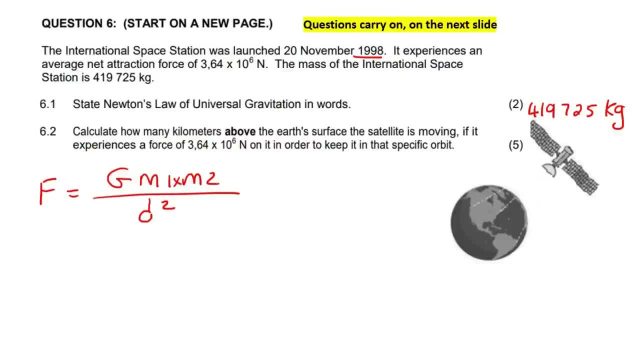 this formula and it helps to trigger the definition. Okay, so let's go get the definition now. So here it is, guys. So every particle in the universe exerts. now, this part might be different to what your teacher says, but you see, 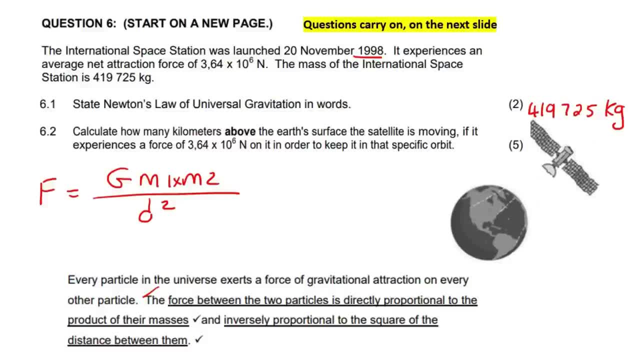 that they're not actually marking you on that first part. The underlying part is where they really care. The force between the two particles is directly proportional to the product of their mass and inversely proportional to the square of the distance between them. Usually this is between: 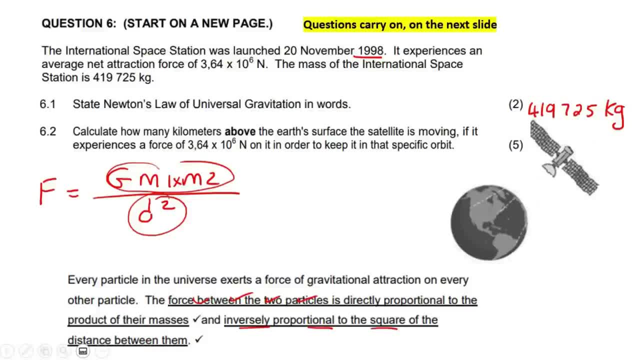 their centers, but you see it changes. It's not exact. Okay, so if you said between their centers, then that's fine. It's only when you are in a specific high school where your teacher thinks that they are the godfather of definitions and their method and their wording is the only way. but that's just silly. 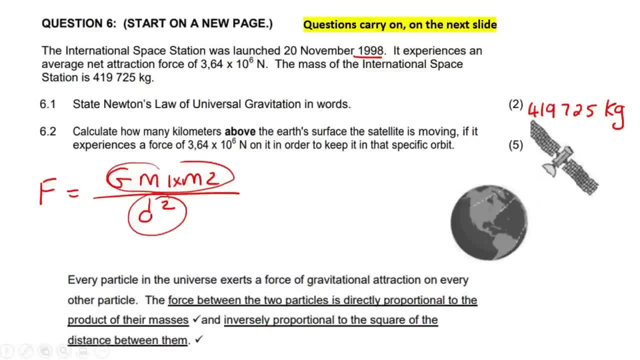 Come on, come on. We live in a big world where everyone's got you know different schools of different, different, different definitions, And so here we have like an official exam paper where you see they're not looking at the first part and your teacher might be like: you need to get that every single part, And don't you? 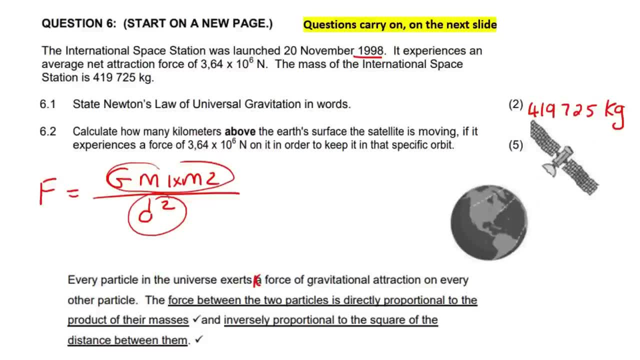 dare leave out the word, the don't you dare and don't Oh don't you leave out that. I think it's so silly, to be honest. But anyways, what can we do? So we can protest, Kevin. Okay, let's not start a rebellion. Yeah, Okay, so 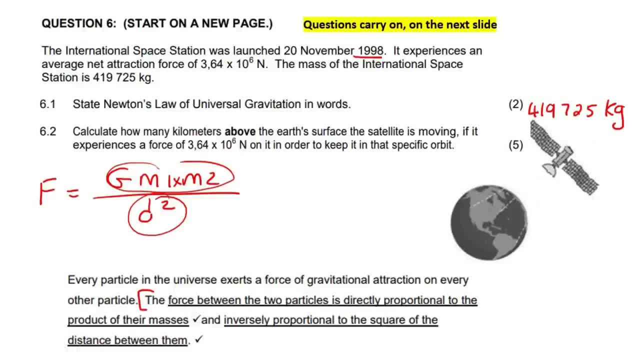 silly man. Okay, so then we just these are the important parts that they're looking for. Okay, I didn't underline this, by the way, this is literally from the memo. they underline that. So that's what they're looking for. They're looking for those key phrases, Okay. So there we go. All right, this. 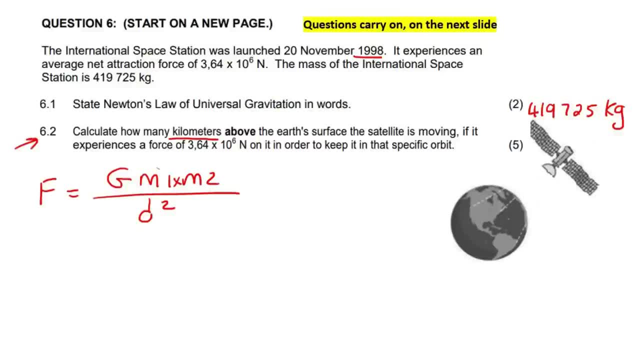 next one says that: calculate how many kilometers. now, here's the key. Here's the key. A lot of learners skip this part. It says above- they were even kind enough to highlight it for you. They saying above: now, Kevin, why does that matter, bro? Because, because, because, because, when you use this formula, 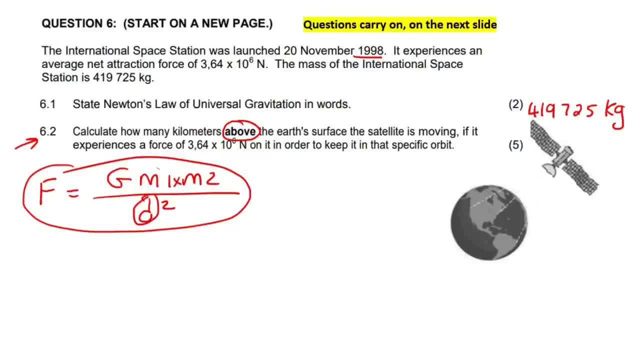 this word is going to be used if, what you, if you, if you're looking for a number, there is a letter that there is a number, that that is to be the number, that is to be the object that you're looking for. It says: from the definition, what did we just say? it is the distance between them. 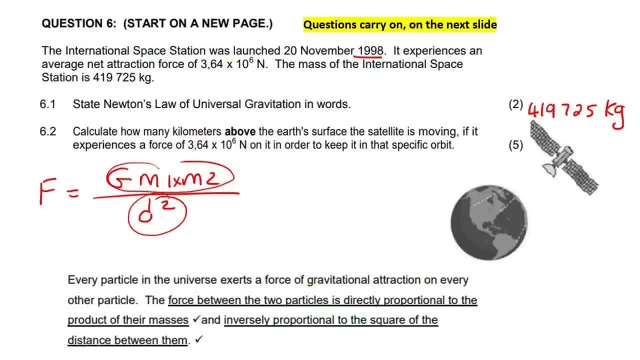 They're looking for those key phrases. Okay, So there we go. All right. This next one says that calculate how many kilometers. Now, here's the key. Here's the key. A lot of learners skip this part. It says above: 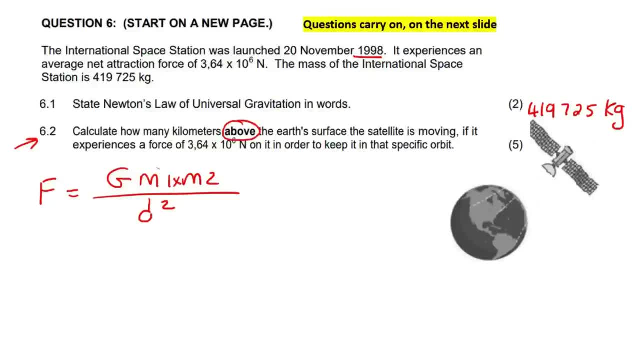 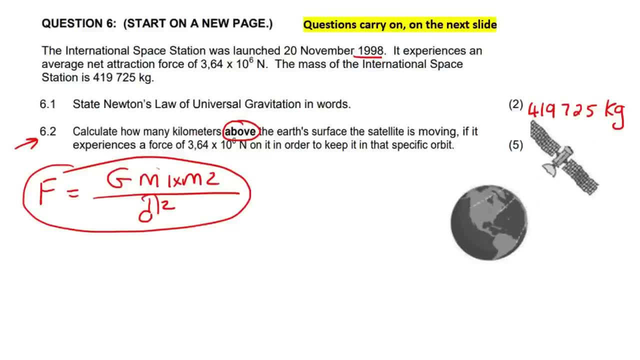 Because, Because, Because, Because This formula This From the definition. what did we just say? It is the distance between them, between the objects, between their centers. That's what it's supposed to say. So here's the center. 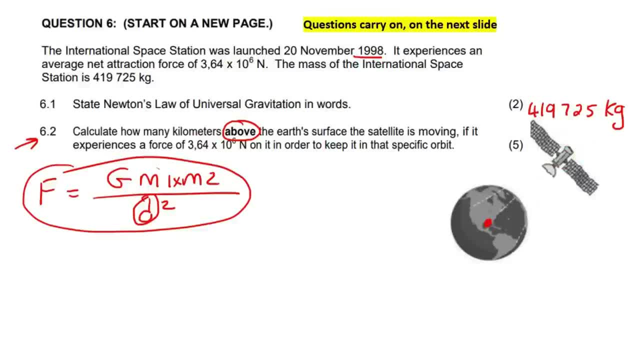 Here's the center, But when it's a little object like this, you can just point over there. It doesn't matter. That is D. Okay, That is not the distance above the earth's surface. The distance above the earth's surface is that part. 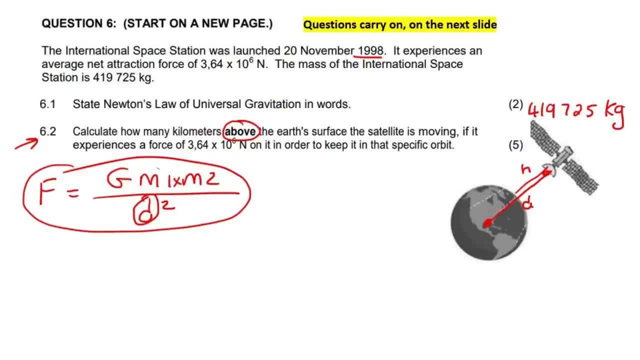 I will just call it H for now. And then you also have this other little distance, which is the radius of the planet. So there are three different distances that you need to keep in mind when you are using this formula is the distance between the objects, which is that it's that distance D that I 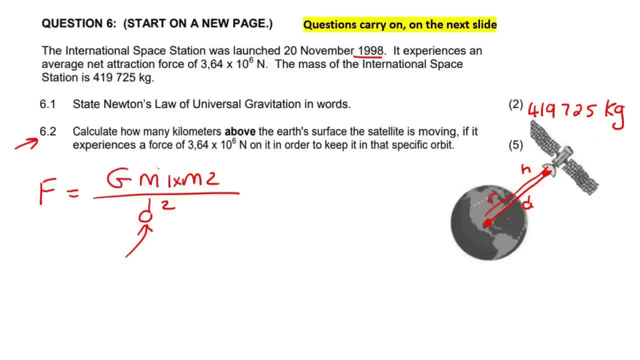 have there. So what are they asking for? If you understand what I'm asking now, what is this distance above the Earth's surface? Which letter is that? Is it R, D or H? Well done, If you said it is H. 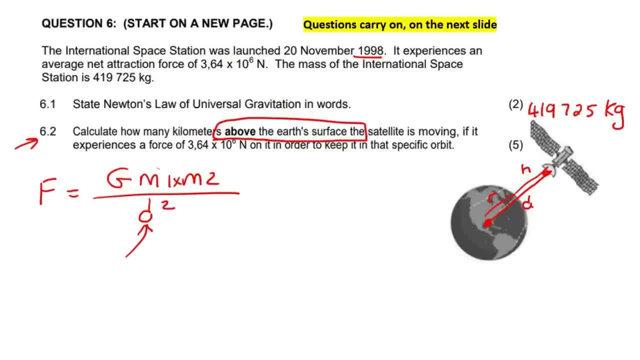 OK, I deserve to. Well, you do. Sorry, I deserve. That doesn't make sense. I need to give you a gold star in your book. Do you guys remember that? Like in grade one, grade two, I used to love that. 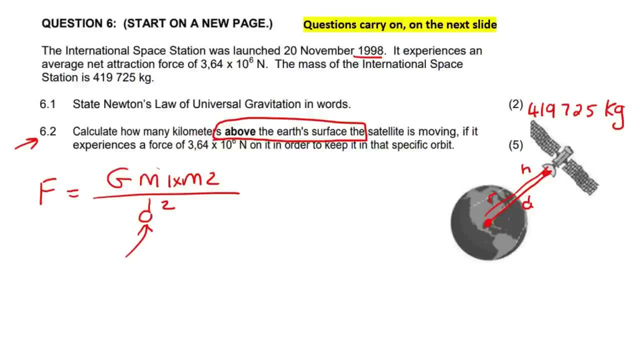 Kevin, can you come to the front please? It's time to mark your work. And then Kevin gets up, walks there, stands next to the teacher's desk- A little bit anxious, to be honest, because some teachers are hella scary. 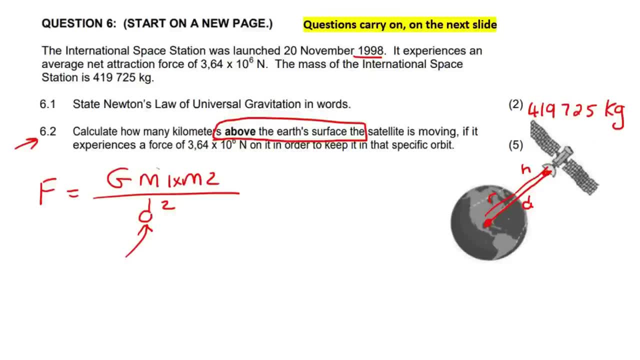 And they like marking your work. And then the teacher looks over her glasses. You know how they do that. My word, But the fear of God. And then they're like good, And then they give you a luminescent green star. 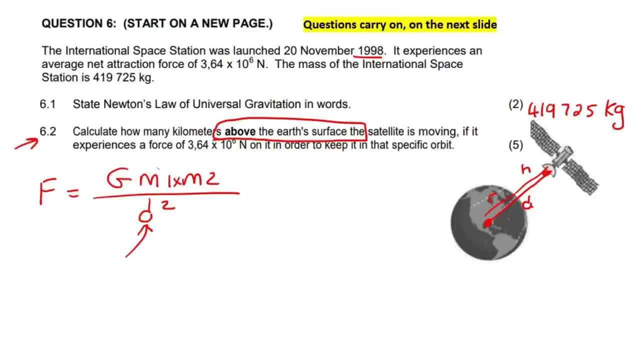 And I'm like, seriously, bro, Is that what my work's worth? What about the gold? And then, yeah, you go sit down with a big smile on your face And your friends are like: did you get a star? 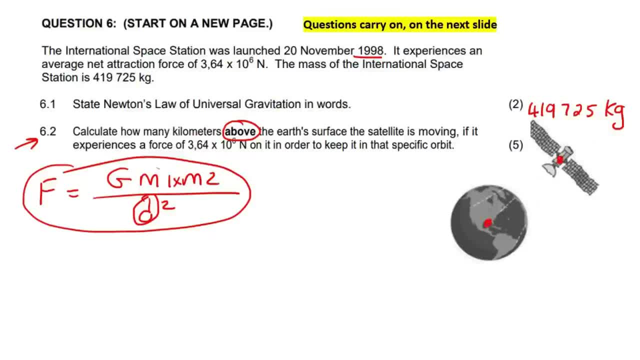 between the objects, between their centers. That's what it's supposed to say. So here's the center, Here's the center. But when it's a little object like this, you can just point over there, It doesn't matter. That is d okay. That is not the distance above the Earth's. 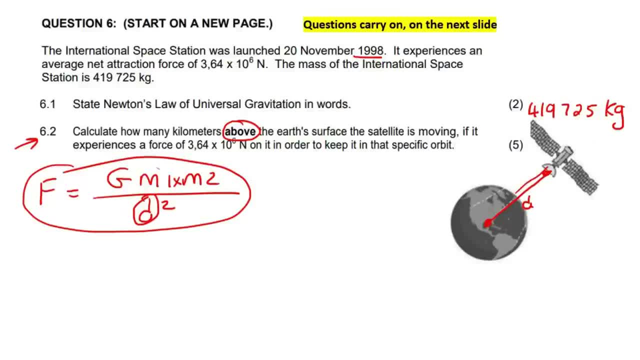 surface. The distance above the Earth's surface is that part. I will just call it h for now. you also have this other little distance, which is the radius of the planet, so there are three different distances that you need to keep in mind when you are using this formula is the distance. 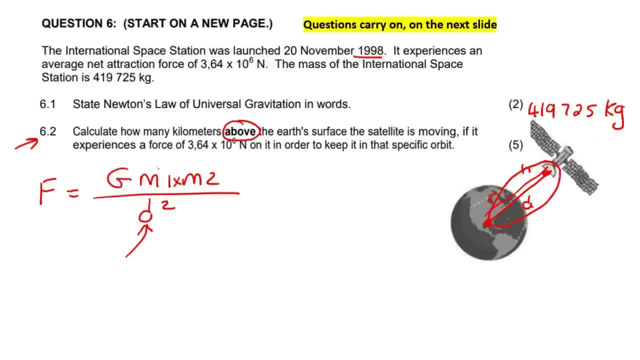 between the objects, which is that it's that distance d that i have there. so what are they asking for? if you understand what i'm asking now, what is this distance above the earth surface? which letters that? is it r, d or h? well done. if you said it is h, okay, i deserve to. well you sorry. 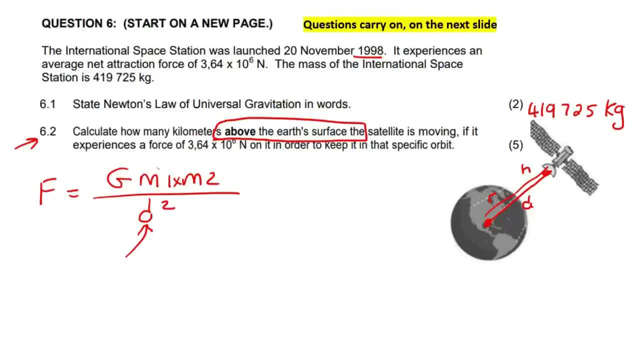 i deserve. that doesn't make sense. um, i need to give you a gold star in your book. do you guys remember that? like in grade one, grade two, i used to love that. kevin, can you come to the front please? it's time to mark your work. and then kevin gets up, walks there, stands next to the teacher's desk. 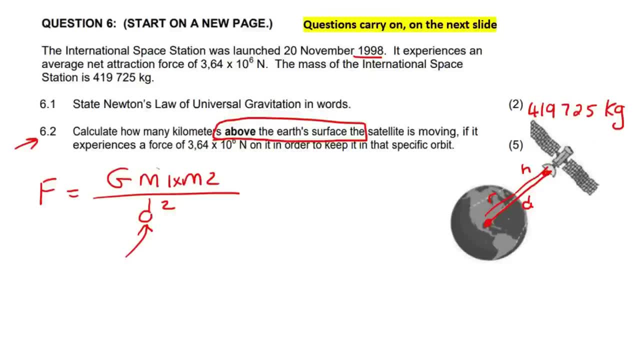 a little bit anxious to be honest, because some teachers are hella scary and i like my, your work. and then the teacher looks over her glasses. you know how they do. that's my word: put the fear of god into us and then they're like good, and then they give you a luminescent green star. 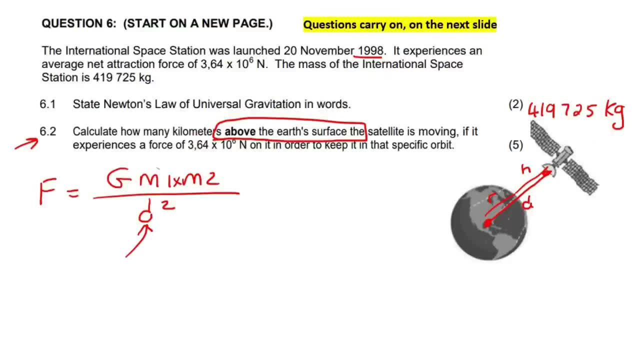 and i'm like, seriously, bro, is that what my worth, my work's worth? what about the gold? and then, and then, yeah, you go sit down with a big smile on your face and your friends are like, did you get a star? and then you're like, yeah, okay, i think i'm extrapolating my story, but i don't. 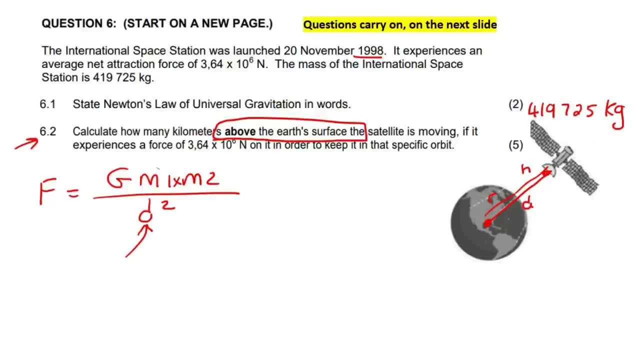 And then you're like: yeah, OK, I think I'm extrapolating my story a bit. I don't think it went exactly like that, But you know, we could keep going on. And so then, suddenly, the girl sitting around me in grade seven, 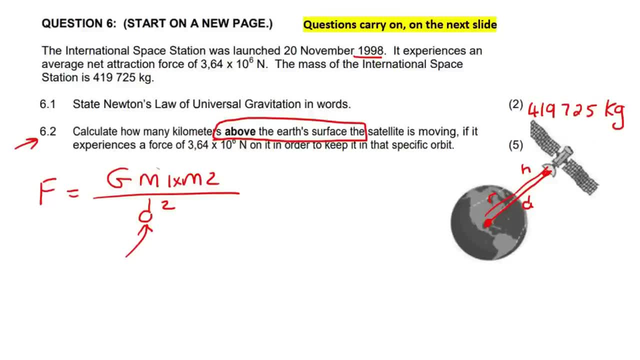 I mean not grade seven, grade one. when I am like seven years old, They're all like, oh, wow guys, he got a star. OK, now I really need to get back to work, OK, so So where were we? 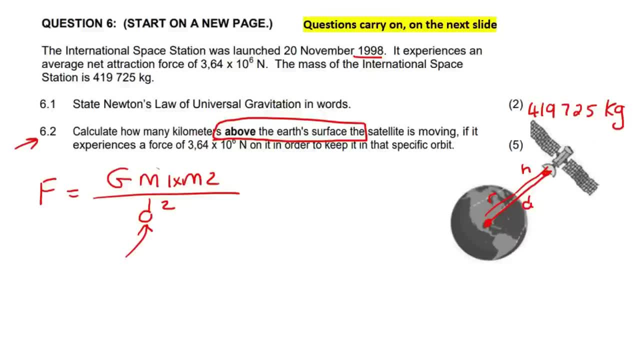 think it went exactly like that. but you know we could keep going on. so then suddenly the girl sitting around me in grade seven- i mean not grade seven, grade one- when i am like seven years old, they're all like, oh, wow, guys, he got a star. okay, now i really need to get back to work, okay, so 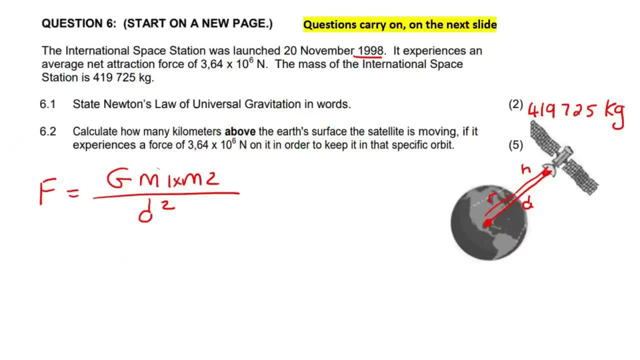 um, so, hmm, uh, where were we okay? so remember, when they say above, please, it's very important that you understand what we're doing here. okay, so the the the to remember is that this formula is the distance between the objects, between, and it's between the centers. but we don't get super technical about the little object, but we do get technical about. 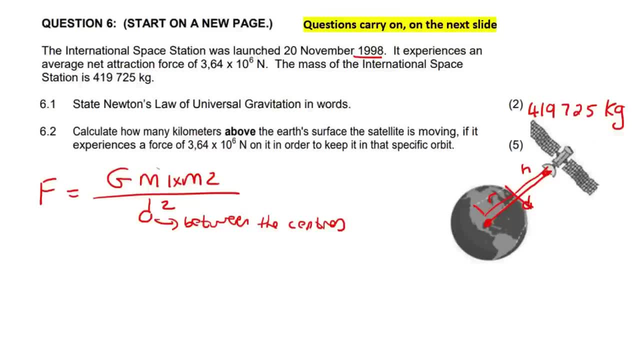 the planet, because a planet's really big. so if you choose the surface and you choose the center, it makes a big difference. but with these objects the center and the surface is like the same thing, so we don't really look at it for those objects, okay, um, if okay. so it says here. 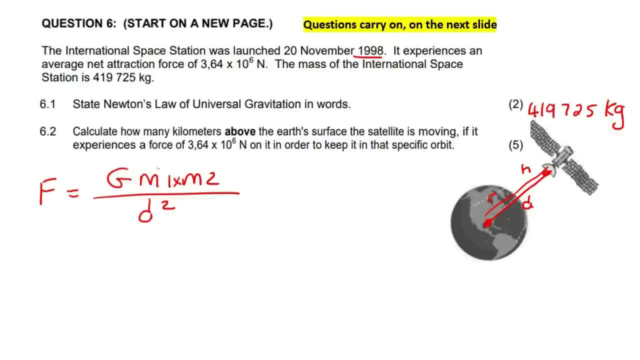 it says: calculate how many kilometers above the if it experiences this force on it, in order to keep it in a specific orbit. and that's also the um, that's also the force that we, we, we had over there, right? so what we will do, ladies and gentlemen, is we will say: um, okay. so we know the force, we know. 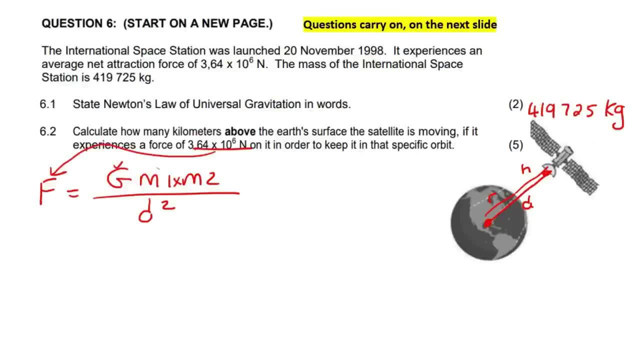 the force, so we can put that over there. g is a constant which we can go grab on our formula sheet and then we can calculate the mass of the two objects, so it's the mass of um, the satellite and earth, and then the d, and then d is the distance between them. so we can go calculate. 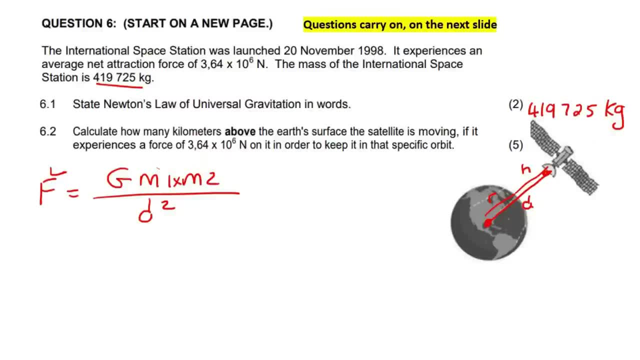 that, because that's the only unknown. uh, but kev, what's the what's like, the um mass of the earth? well, and what's g? okay, now, luckily some people don't know this, but i didn't when i was in high school, but on the formula sheet um, this bra sitting here had to memorize all the stuff. 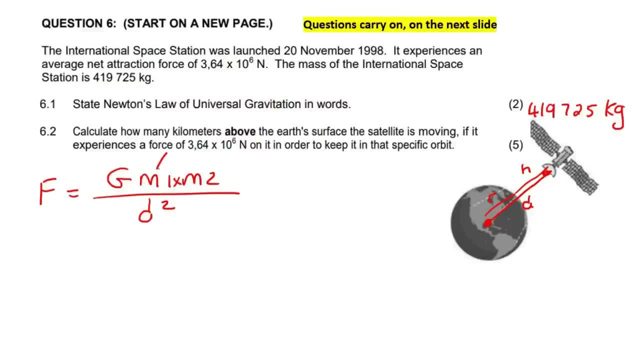 but on the formula sheet they do give you um the mass of planet earth and they also give you um the mass, i mean the radius. uh, well, this isn't the radius, but we might need that. we will need that later, but on the formula sheet they actually 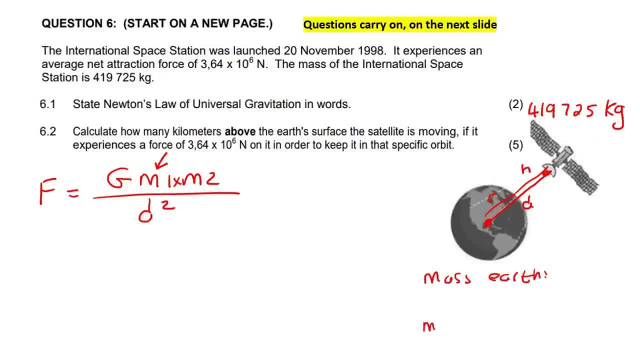 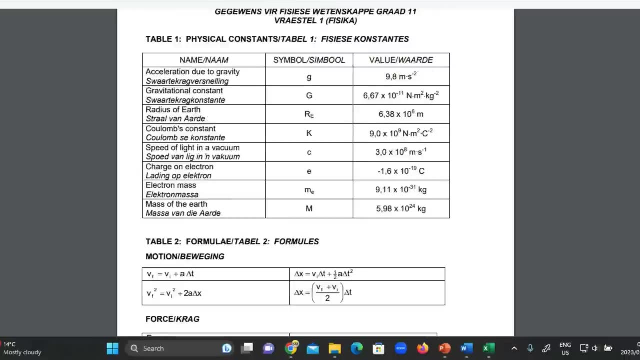 give us the mass of earth and then the mass. why am i keep saying the mass of the radius? who's this guy? so then the radius of earth. that is actually on your formula sheet. let me go show you, okay. so here we are on the formula sheet now. can you see? in row number two there's the capital g over there. 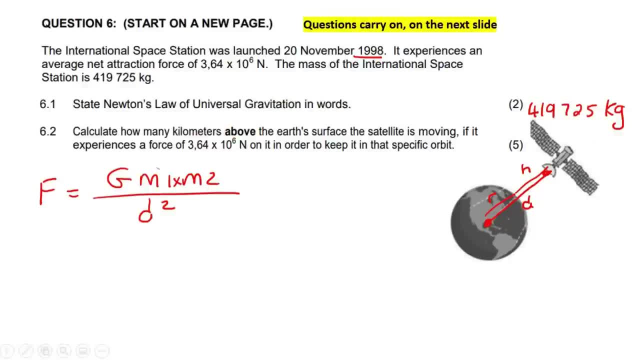 OK, so remember when they say above, please, it's very important that you understand what we're doing here, OK, so the main thing to remember is that this formula is the distance between the objects, between, and it's between, the centers. But we don't get super technical about the little object, but we do get technical about the planet, because a planet's really big. 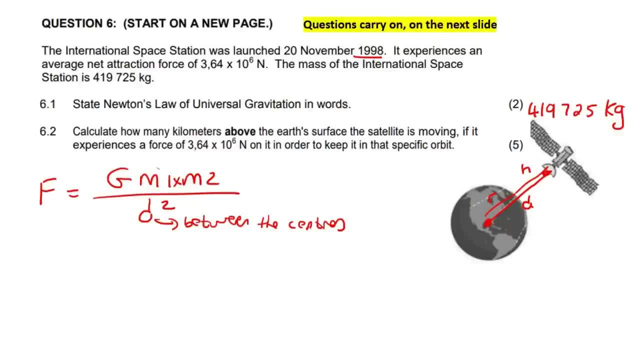 So if you choose the surface and you choose the center, it makes a big difference. But with these objects the center and the surface is like the same thing, So we don't really look at it for those objects, OK, if OK. so it says here. 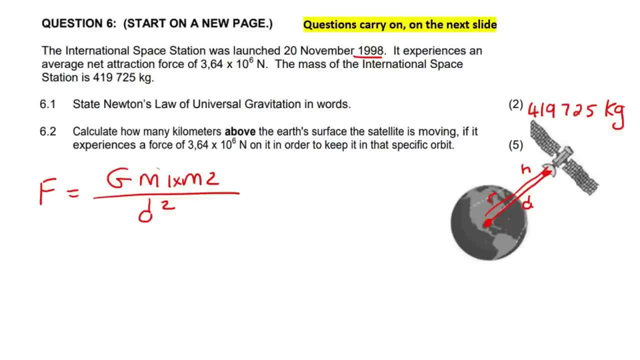 It says, calculate how many kilometers above the data data, if it experiences this force on it In order to, In order to keep it in a specific orbit. And that's also the, that's also the force that we, we, we- had over there. 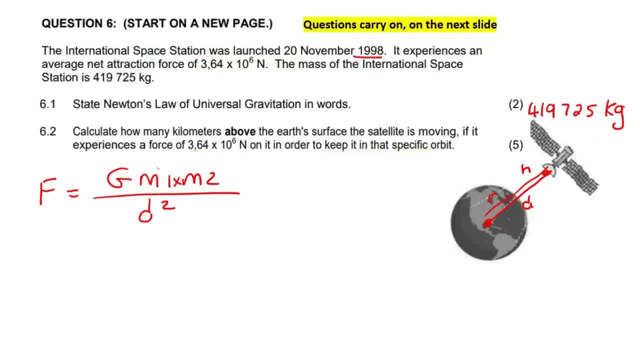 Right. So what we will do, ladies and gentlemen, is we will say: OK, so we know the force, We know the force, So we can put that over there. G is a constant which we can go grab on our formula sheet. 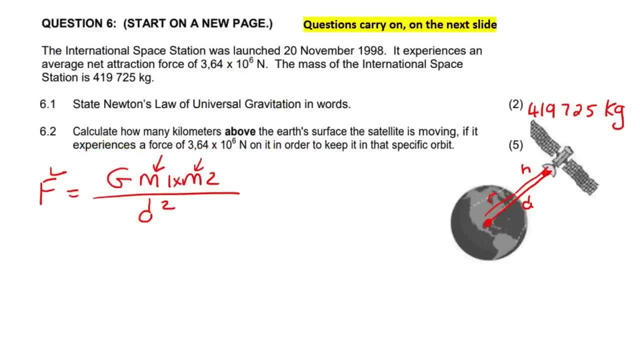 M is the mass of the two objects, So it's the mass of the satellite and Earth, And then the D, and then D is the distance between. So we can go calculate that, because that's the only unknown. But, Kev, what's the what's like the mass of the Earth? 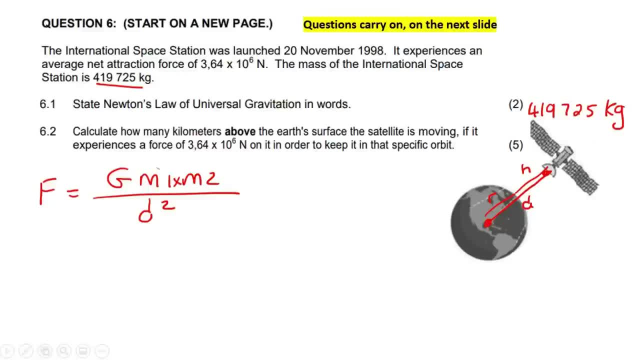 Well, and what's G? OK now, luckily some people don't know this, but I didn't when I was in high school. But on the formula sheet, this bra sitting here had to memorize all the stuff. But on the formula sheet they do give you the mass of planet Earth. 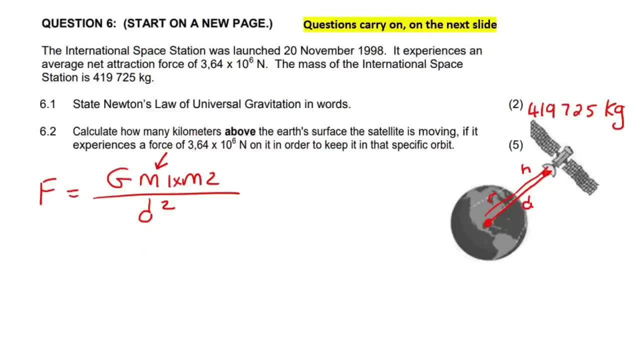 And they also give you the mass. I mean the radius- Well, this isn't the radius, but we might need that And we will need that later. But on the formula sheet they actually give us the mass of Earth and then the mass. 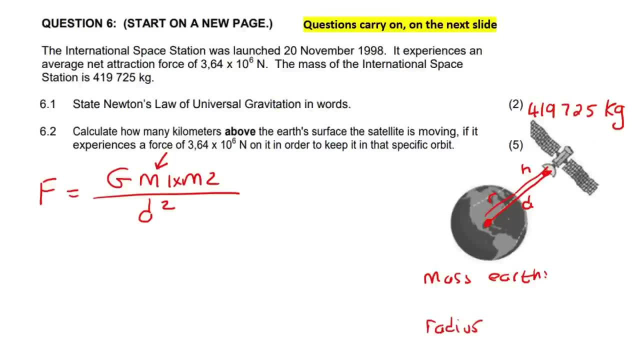 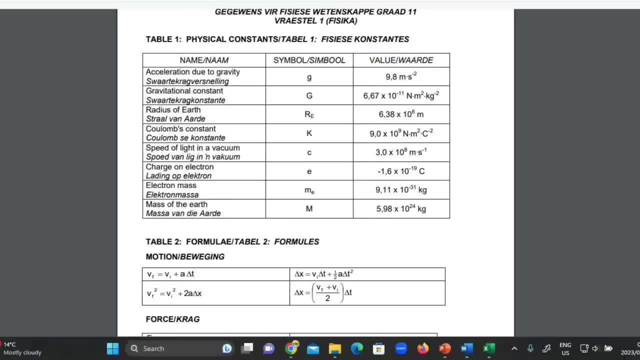 Why am I keep saying the mass of the radius? Who's this guy? So then the radius of Earth. that is actually on your formula sheet. Let me go show you. OK, so here we are on the formula sheet. Now. can you see? in row number two there's the capital G over there. 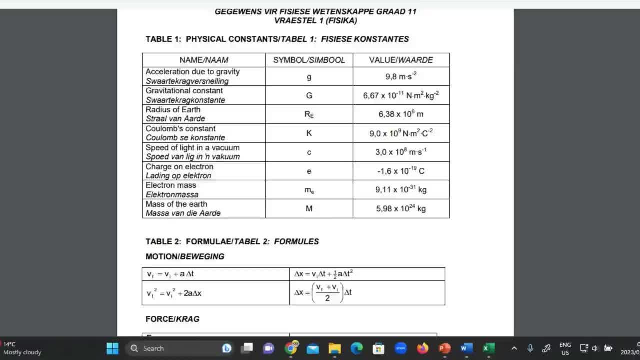 So that is, that's the G that we're looking for. And then if we go down, down, down, down, down to- Oh yeah, Um, Mass of Earth, Can you see it? Mass of Earth is M, And then you can see radius of Earth, which is RE. 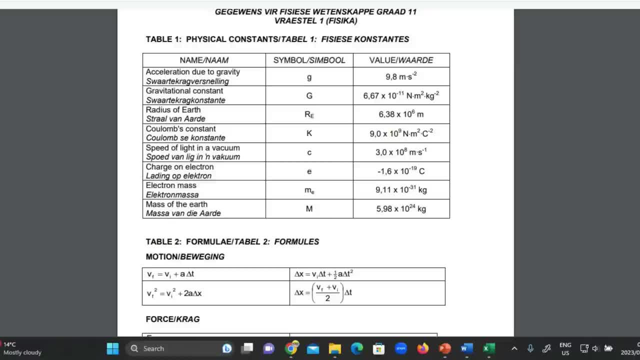 um, that's the g that we're looking for. and then if we go down, down, down, down down to- oh yeah, um, mass of earth, can you see it? mass of earth is m, and then you can see radius of earth, which is r, e. okay, so i forgot about that. one radius of earth, mass of earth, how cool is that? so i'm just 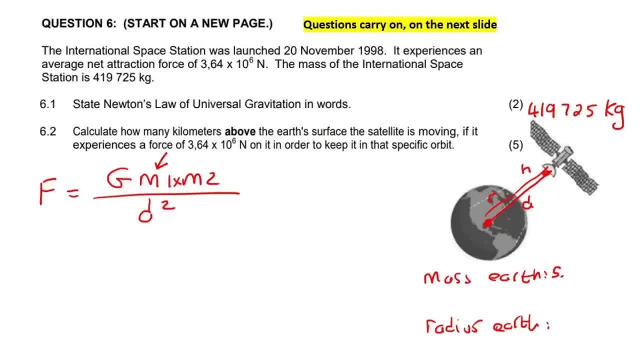 write this down. so long i'm going to do the same, okay. so earth's mass was 5.98 times 10 to the 24. kilograms, and then the radius of the earth was 6.38 times 10 to the 6th. 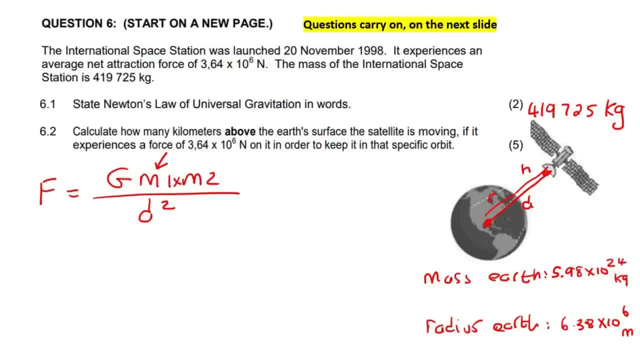 and that was in metres. okay, so, but remember that that is the radius of the earth, so that's just little r, okay. so let's ignore that part for now. let's go fill everything in. so 3.64 x 10 to the six g- i didn't write that one down, but you guys remember- 6.67 times ten to the negative 11.. 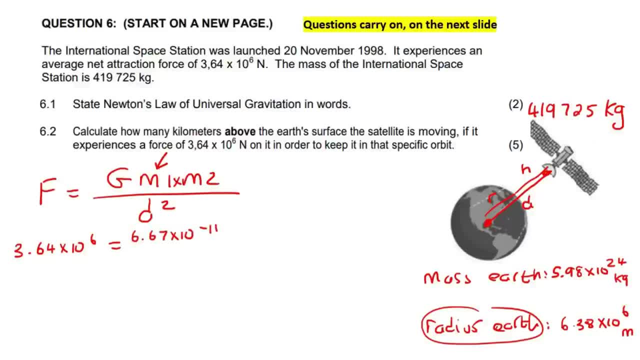 I know the IEB. I think it's a little different. I think it's like 6.6 or 6.7.. So just look out for that. And then mass of the first object. So it doesn't matter, We can use the ISS or IS squared, International Space Station. 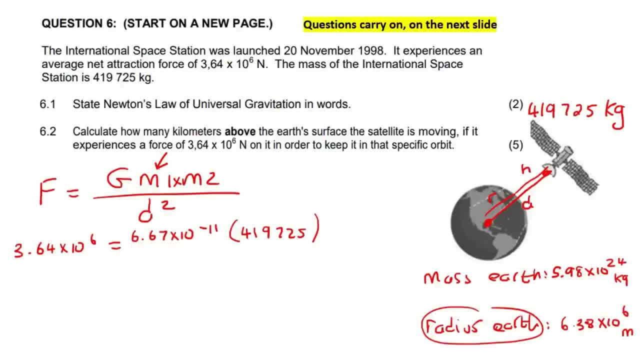 Yo, what up. what up? 4, 1,, 7, 2, 5.. Kevin, you're so stupid bro, I know. And then the mass of the other object, which is Earth itself, which is 5.98 times 10 to the 24.. 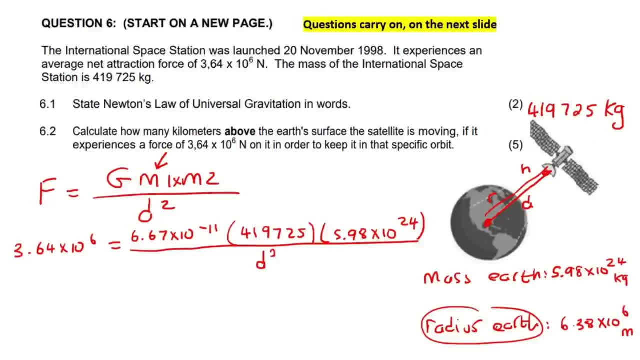 And then the distance we don't know. So we'll just say D squared. Now, to get the D squared by itself, you're just going to take it and do cross multiplication over there, And then you're going to take this one and divide it back down. 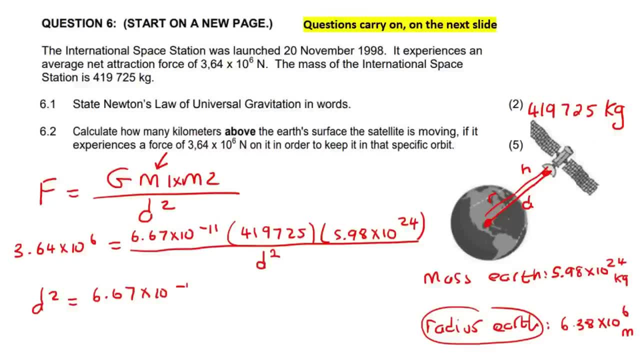 So you're going to end up with this, Okay, Okay, And then, of course, together, If you get D alone, you would have to take the square root. So go, have fun typing those 50 million numbers into your calculator. 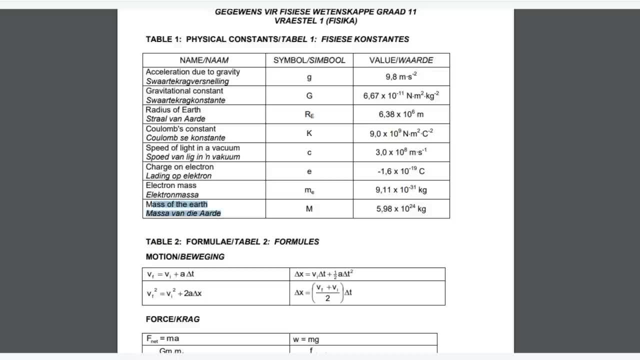 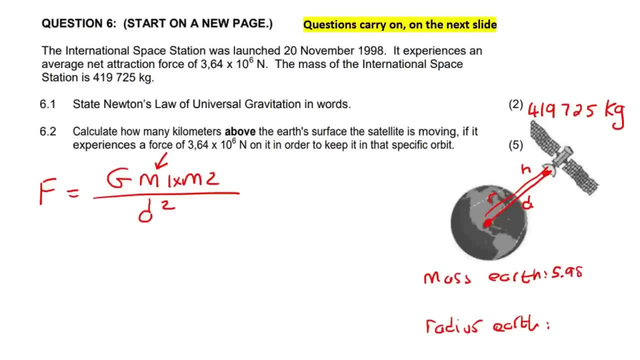 OK, so I forgot about that. one Radius of Earth, mass of Earth- How cool is that? So I'm just write this down so long I'm going to do the same. OK, so Earth's mass was five point nine, eight times ten to the twenty four kilograms. 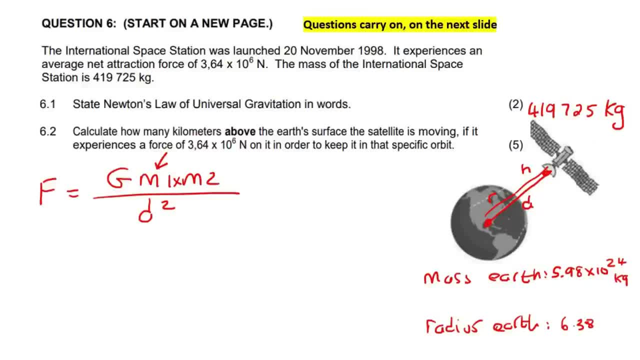 And then the radius of the Earth was six point three, eight times ten to the six, And that was in meters. OK so, but remember that that is the radius of the Earth. so that's just little R, OK, so let's ignore that part for now. 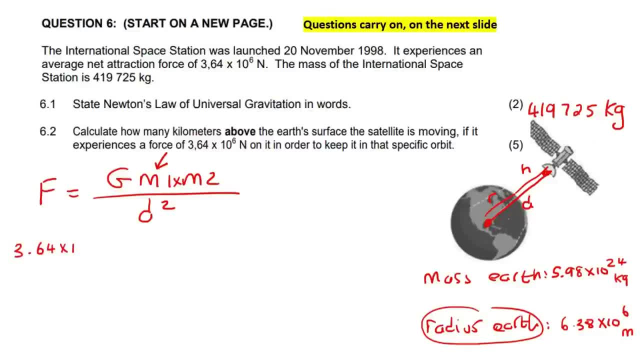 Let's go fill everything in. So three point six, four times ten to the six G. I didn't write that one down but you guys remember six point six, seven times ten to the negative eleven. I know the IEB, I think it's a little different. 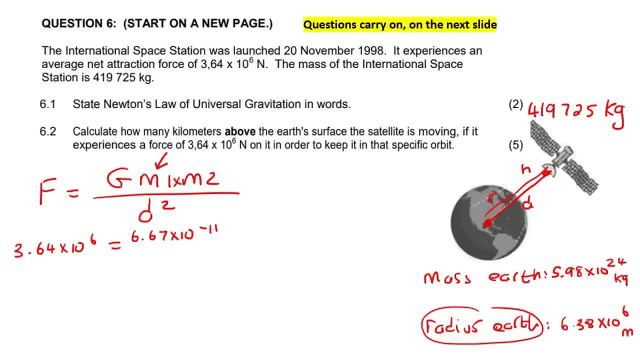 I think it's like six point six or six point seven. So just look out for that, And then mass of the first object. So it doesn't matter, We can use the ISS or ISSquared International Space Station. 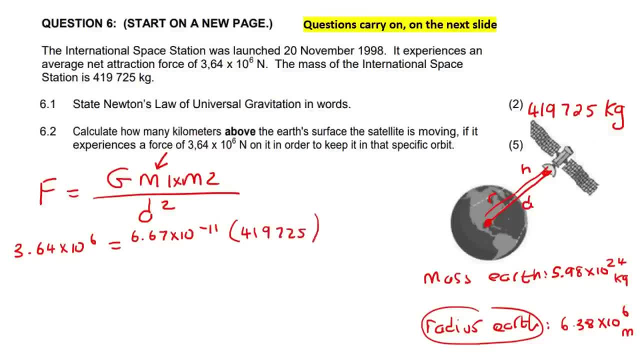 Yo, what up? what up? four, one, seven, two, five- Kevin, you're so stupid bro, I know- And then the mass of the other object, which is Earth itself, which is five point nine, eight times ten to the twenty four. 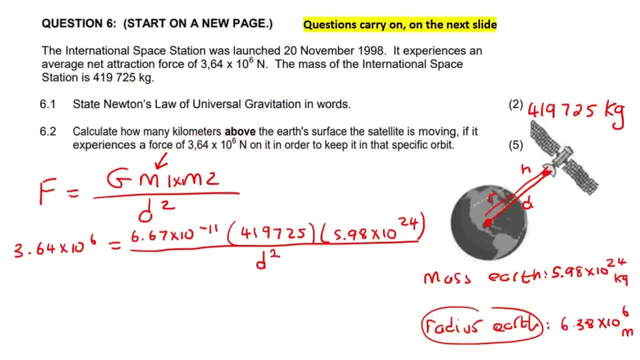 And then the distance we don't know. So we'll just say D squared. Now, to get the D squared by itself, you're just going to take it and do cross multiplication over there, And then you're going to take this one and divide it back down. 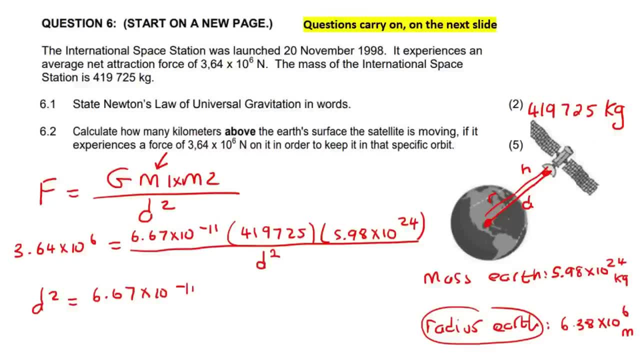 So you're going to end up with this, OK, and then, of course, to get D alone, you would have to take the square root to go. have fun typing those 50 million numbers into your calculator, And so we end up with the distance. 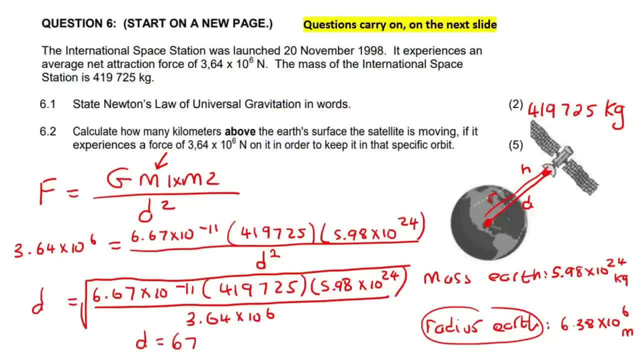 As six, seven, Eight, one, eight, oh four point zero, three, And that's still in meters. OK, now that's this distance over here, But they want H. But can you see that the radius Plus the H, which is the height above the surface, is the same as the distance? 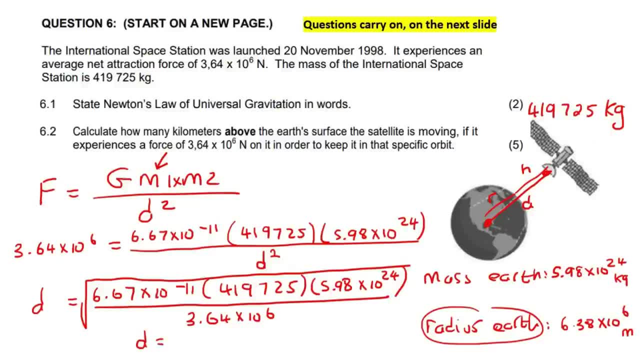 And so we end up with the distance as 6,, 7,, 8,, 1,, 8,, 0,, 4,, 0.3.. And that's still in meters. okay, Now, that's this distance over here, but they want H. 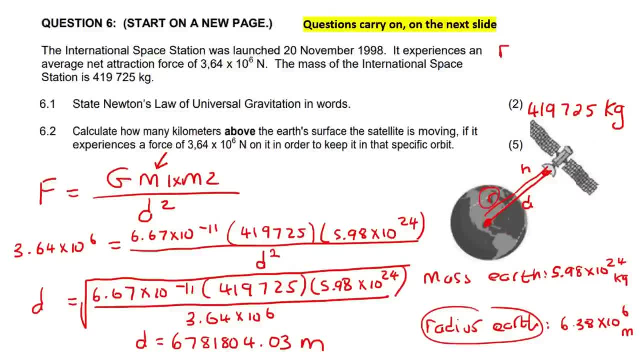 But can you see that the radius plus the H, which is the height above the square surface, is the same as the distance. So now they wanted H. I've just called it H, right? It's not actually called H. So to get H. okay now, this is a bit of an interesting formula. 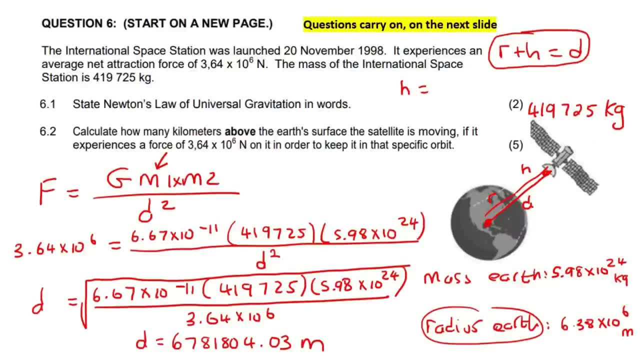 Now you've got to think carefully, Like: how do you get H alone? Okay, guys, I'm just pulling your leg, You just take R to the other side, Okay. And so now we can actually just go work out H, because we know the distance as 6, 7,, 8,, 1,, 8,, 0,, 4,, 0,, 3.. 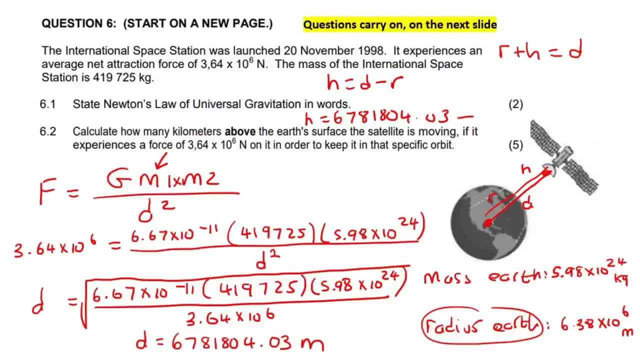 Subtract the distance, So sorry, subtract the radius of the Earth, which is this one over here, 6.38 times 10 to the 6.. And if we work this out now, we end up with 4, 0,, 1,, 8.. 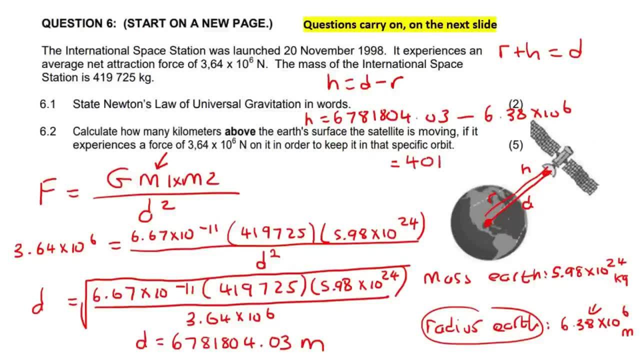 Well, okay, let's write it a little bit better. People at home aren't sitting with microscope, Microscopes 0.03.. Now, that's in meters, but they said in kilometers, So just divide that by 1,000.. 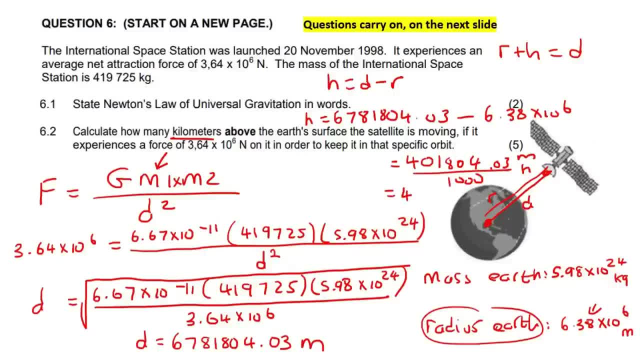 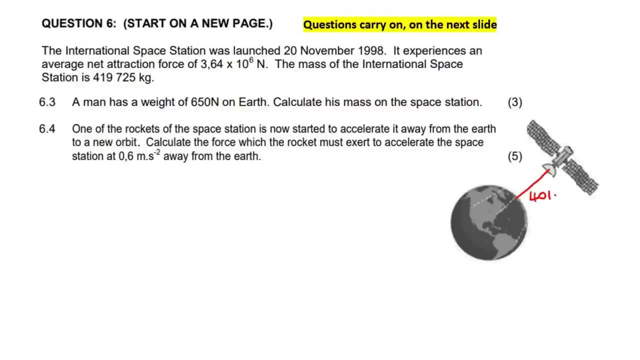 So we'll divide that by 1,000. And we get 401.80.. And that'll now be in kilometers. Okay, so in the previous question we worked out that this distance here was 401.80 kilometers. This one says that a man has a weight of 650 newtons on Earth. 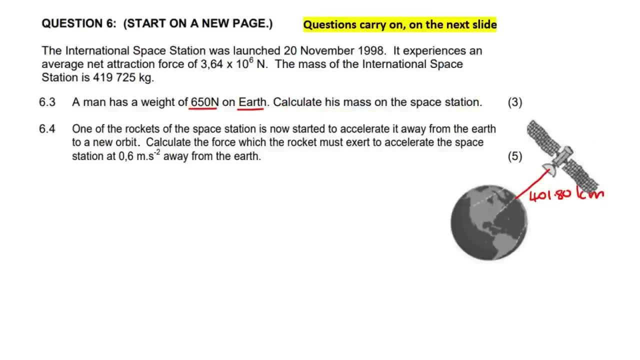 Calculate his mass on the space station? Really easy question, Because we know that mass on Earth and the mass at the International Space Station should be exactly the same. Mass never changes. Think about it If you are on Earth and you go to the International Space Station and you look at your two arms. 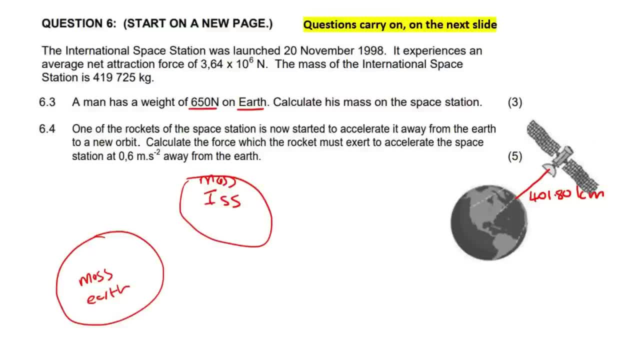 if you had two arms on Earth, you'll still have two arms on the International Space Station. So you haven't lost bones, You haven't lost muscle, You haven't lost anything. So mass never changes. But, Kevin, I thought you become lighter. 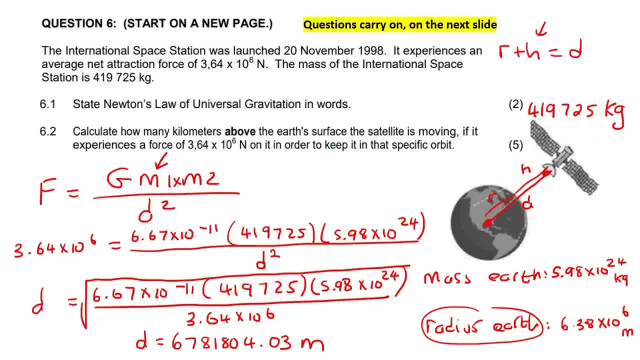 So now they wanted H. I've just called it H, Right, It's not actually called H. So to get H. OK. now, this is a bit of an interesting formula. Now you've got to think carefully, Like, how do you get H alone? 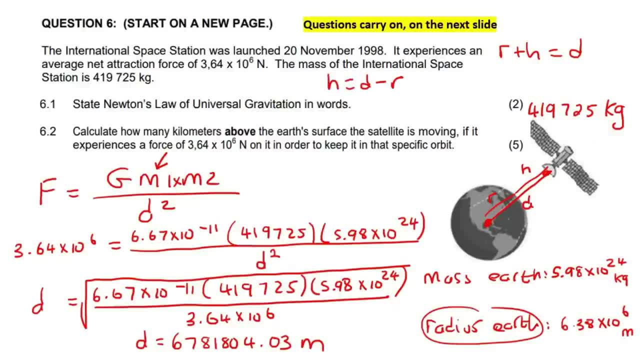 OK guys, I'm just pulling your leg, You just take R to the other side. OK, and so now we can actually just go work out H, because we know the distance as six, seven, eight, one, eight, oh, four point zero, three. 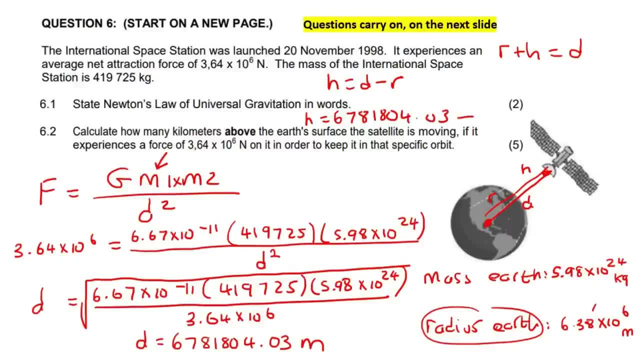 Subtract the distance, So sorry, subtract the radius of the Earth, which is this one over here: Six point three, eight times ten to the six, And if we work this out Now, we end up with four, oh one, eight. Well, Kev, let's write it a little bit better. 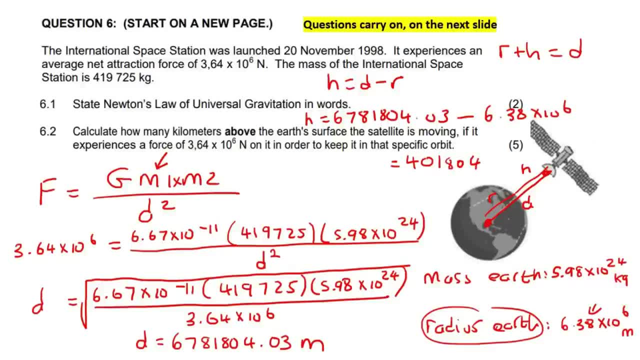 People at home aren't sitting with microscope. Microscopes, point oh three. Now that's in meters, but they said in kilometers. So just divide that by one thousand, So we'll divide that by one thousand, and we get four hundred and one point eight zero. 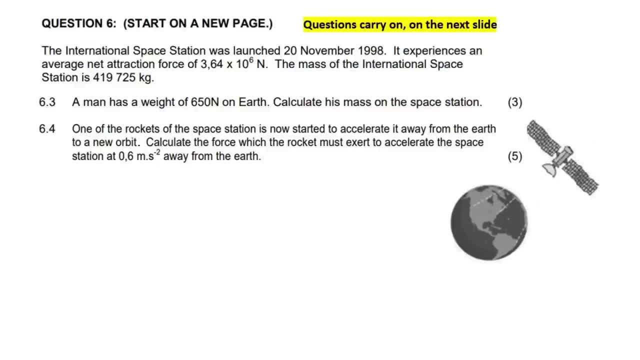 And that'll now be in kilometers. OK, So in the previous question We worked out that this distance here was four hundred and one point eight zero kilometers. This one says that a man has a weight of six hundred and fifty Newtons on Earth. 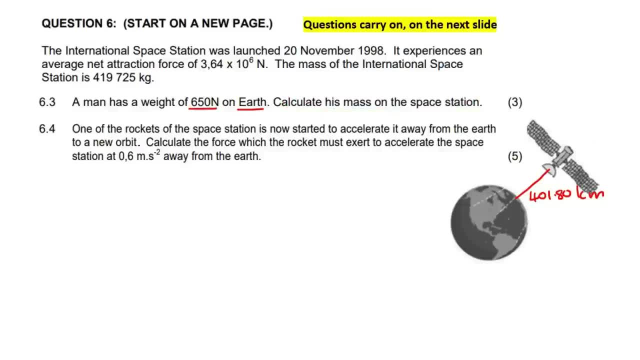 Calculate his mass on the space station? Really easy question, because we know that mass On Earth And the mass at the International Space Station Should be exactly the same. Mass never changes. Think about it If you are on Earth and you go to the International Space Station and you look at your two arms. 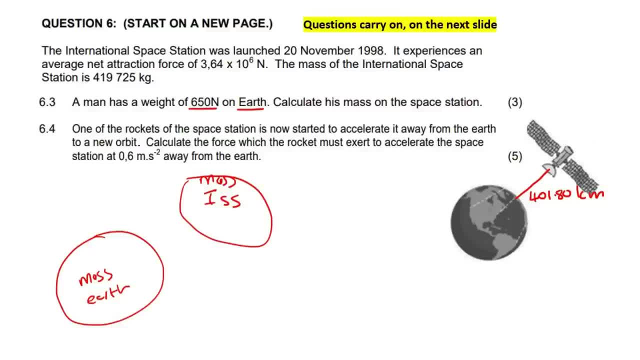 If you had two arms on Earth, you'll still have two arms on the International Space Station. So you haven't lost bones, You haven't lost muscle, You haven't lost anything. So mass never changes. But, Kevin, I thought you become lighter. 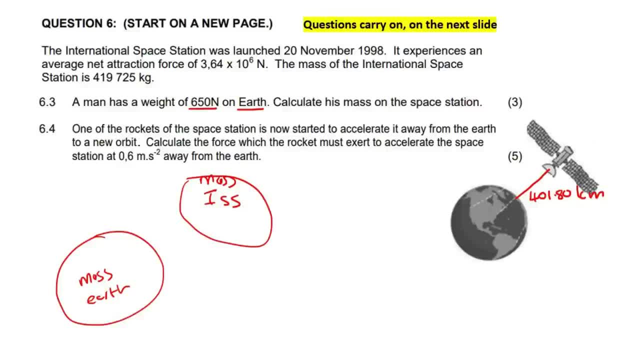 Yes, that is your weight. That's a different thing. We talk about mass, Mass and weight. The confusion is because in real life we talk about mass and weight like they're the same, but they're not. in science and physics, Mass and weight are two different things. 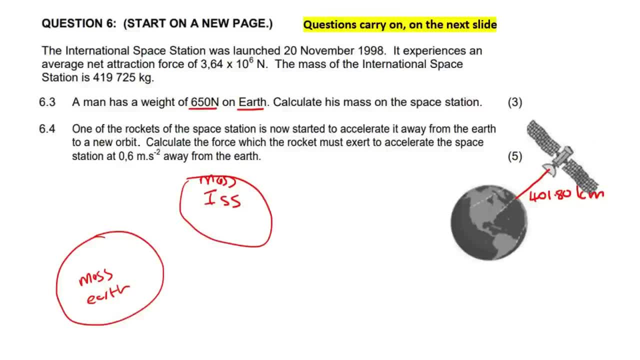 Yes, that is your weight. That's a different thing. We talk about mass and weight. The confusion is because in real life we talk about mass and weight like they're the same, but they're not. In science and physics, mass and weight are two different things. 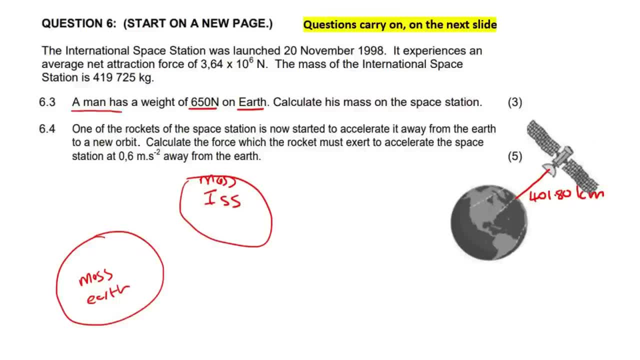 So what this means is that if we can work out the person's mass on Earth, then we know what the person's mass on the space station will be. So we know that to calculate weight on Earth you would use MG, or on any planet actually, you'd use MG. 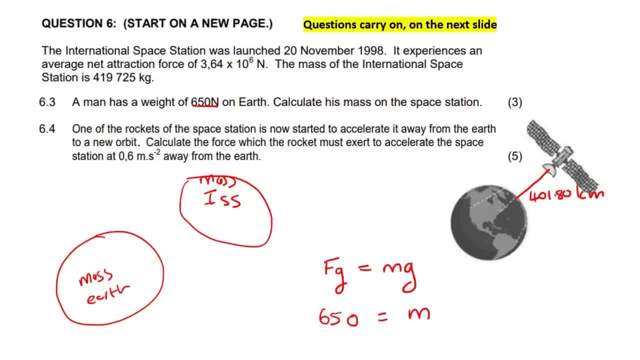 Now we know that this person's weight is 650.. We don't know what their mass is And we know that on Earth we can use 9.8.. On a different planet you would use a different number. Now, if you had to go calculate the mass, you would get 66.33 kilograms. 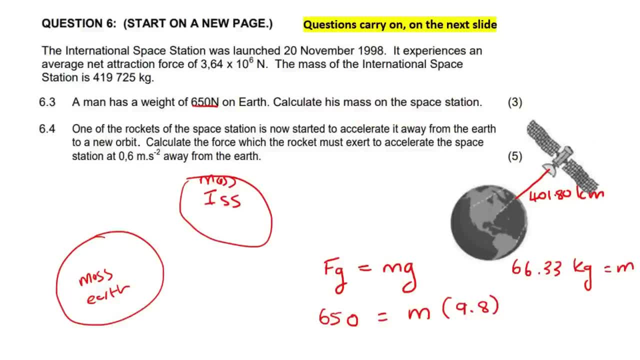 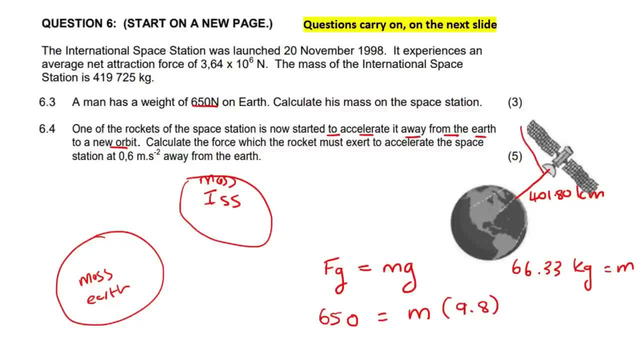 So that's the mass. So they start it up And what that does is it starts accelerating the space station away from Earth. Okay, Calculate the force that the rocket must exert to accelerate the space station at that acceleration away from the Earth. Okay, so this is definitely just going to be an Fnet. equals to MA. 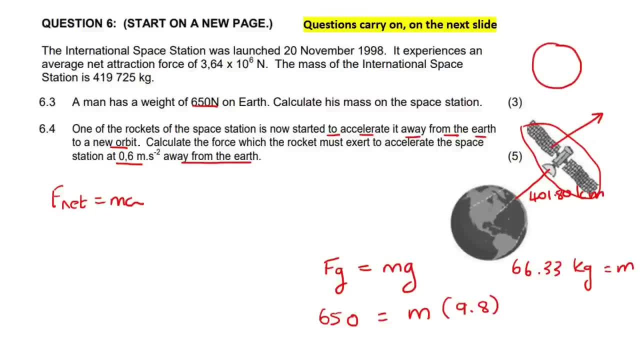 Okay Now, if you look at Earth, I'm going to draw it like this, rather- And if you look at the space station, there is already a force. If you had to do a force, you would have to do a force. 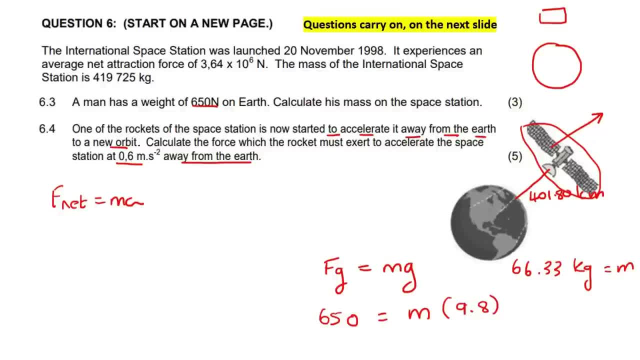 Now remember, if you have a force here, just do a force. You would be doing a force by doing carbon dioxide. so a free body diagram acting on the space station. What there's going to be now is there's going to be a force of gravity. 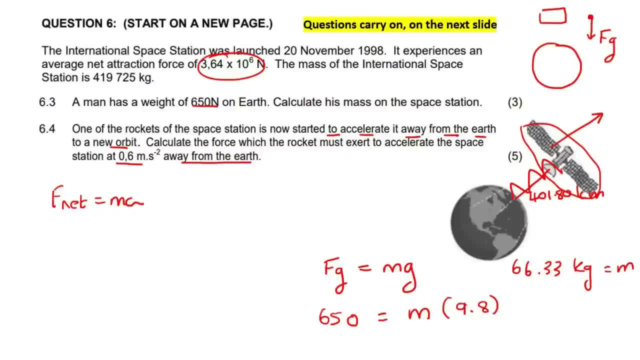 which we already know, is this one over here, at that distance away. And then what it's going to do now is it's going to switch rockets. It's going to switch one of the rockets on, So F our safe applied. Okay, so it's going to put one of those rockets on. 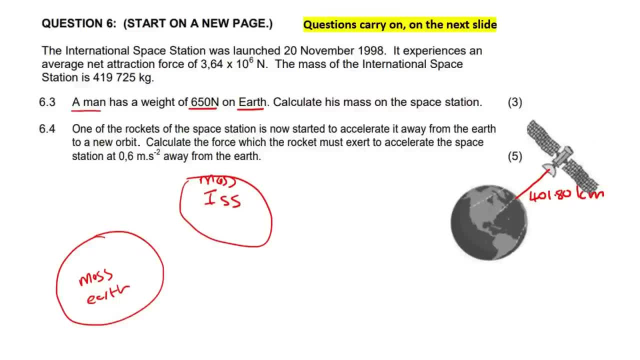 So so. so what this means is that if we can work out the person's mass on Earth, then we know what the person's mass on the space station will be. So we know that to calculate weight on Earth, you would use MG on any planet. 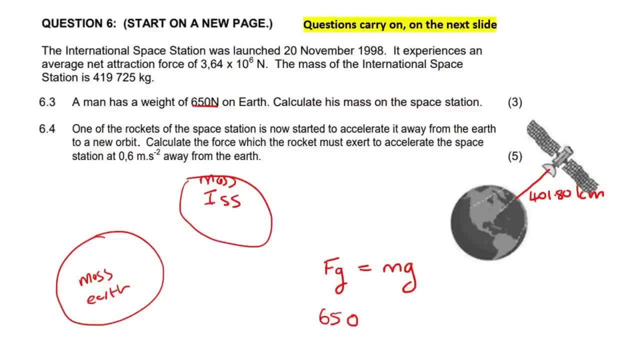 Actually, you'd use MG. Now we know that this person's weight is 650.. We don't know what their mass is and we know that on Earth we can use 9.8. on a different planet, you would use a different number. 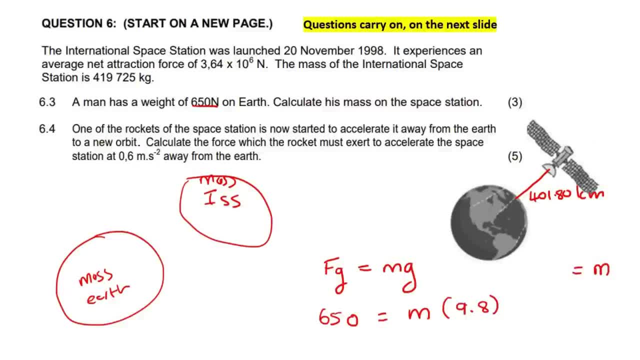 Now, if you had to go calculate the mass, you would get 66.33 kilograms. Now that is the mass, And so that will also be the mass on the space station. One of the rockets in the space station is now started to accelerate. 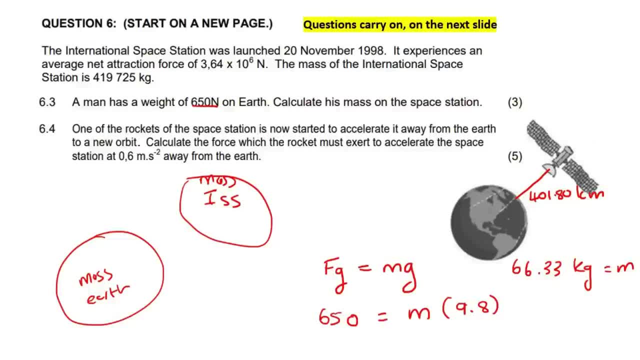 Wait, one of the rockets of the space station has now started to accelerate. It's away from the Earth to a new orbit. Wait, wait, one of, Oh, OK, one of the rockets of the space station is now started. OK, why? to accelerate it away from the Earth to a new orbit? 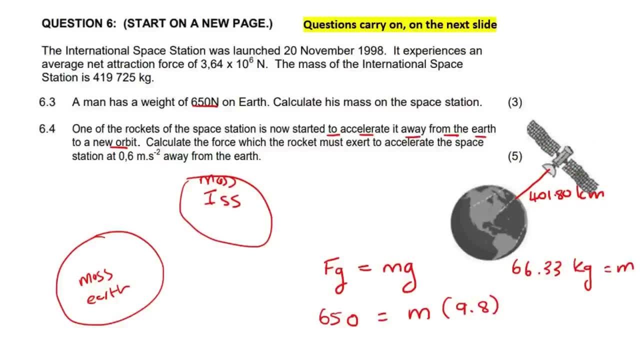 OK, so there is the space station and it's got a rocket. OK, one of the rockets has started, So they, they, they started up, And what that does is it starts accelerating the space station away from Earth. OK, calculate the force that the rocket must. 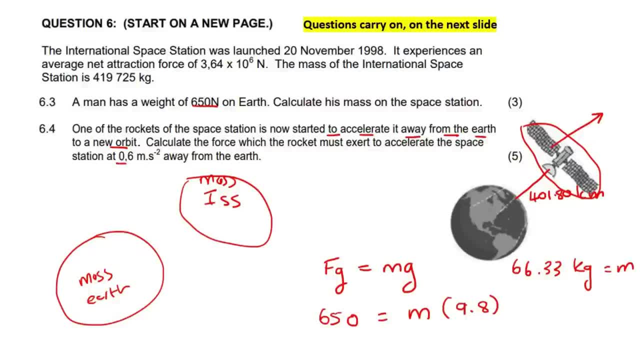 Exerts to accelerate the space station at that acceleration away from the Earth. OK, so this is definitely just going to be an F net equals to MA. OK, now, if you look at Earth, I'm going to draw it like this rather: 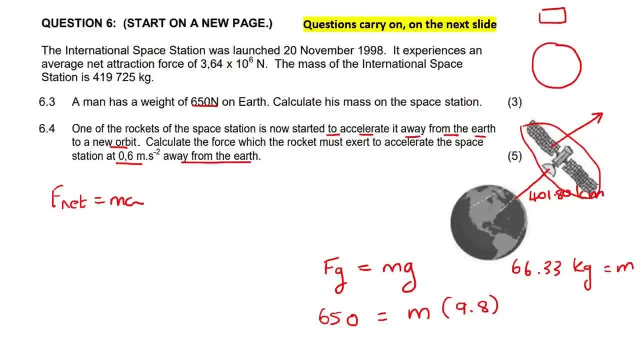 And if you look at the space station, there is already a force. If you had to do a free body diagram acting on the space station, what there's going to be now is there's going to be a force of gravity, which we already know is sorry. 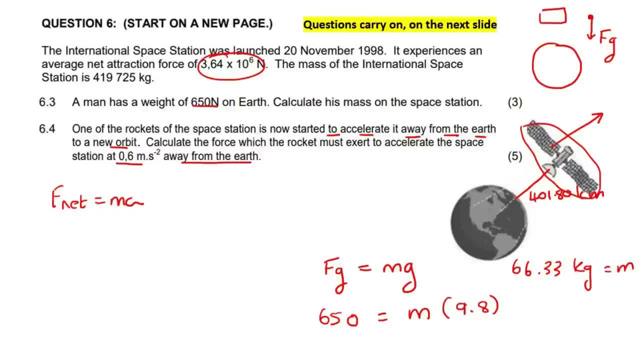 Not, there is this one over here, at that distance away. And then what it's going to do now is it's going to switch rockets. It's going to switch one of the rockets on. So if I say F applied, OK, so it's going to put one of those rockets on. 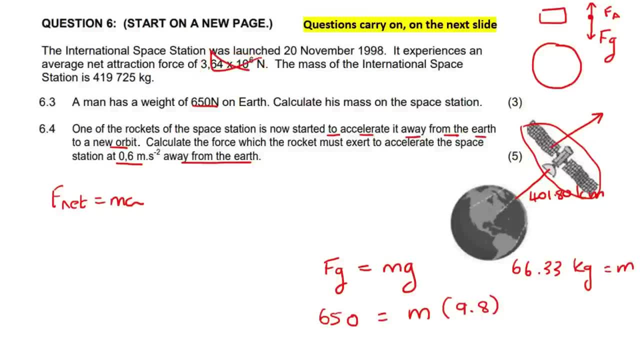 OK, so remember: your F net is not going to be this number anymore. Your F net is going to be the combination of these two. So let's just go say that the F net will now be a less choose going away from the Earth as positive. 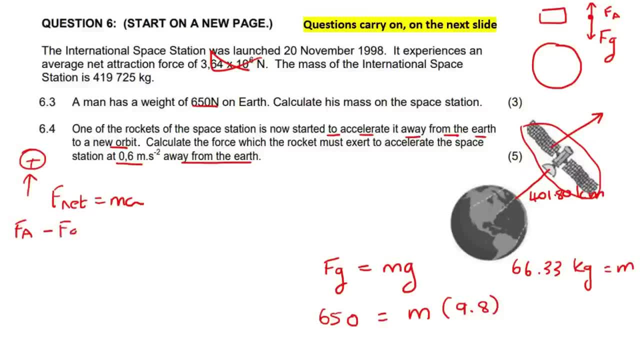 So let's say the applied force of the rocket Minus The gravitational acceleration, which is still going to be that at that same distance. Right, Because as the rocket gets switched on it's still at the same distance, So we can still use that value. and then we can use the mass of the object. 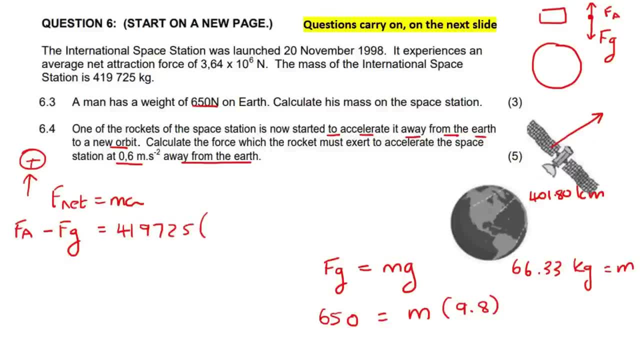 It's always the object, which is four, one, nine, seven, two, five, And the acceleration that we are going for is zero point six. So we can then say that the applied force take away three point six, four times ten to the six, is equal to all of this. 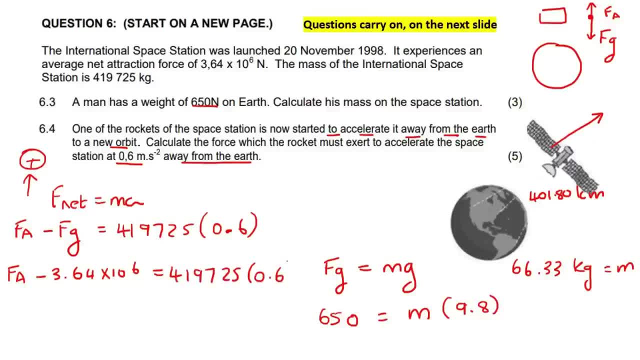 And so if we're to go work out the applied force, we'd end up with three, eight nine, one, eight, three, five Newtons. So that is the force that one of those rockets would have to exert to cause that zero point six acceleration. And because it is a force, it's a vector. 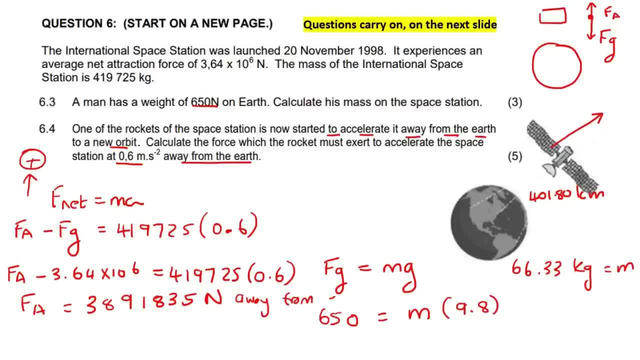 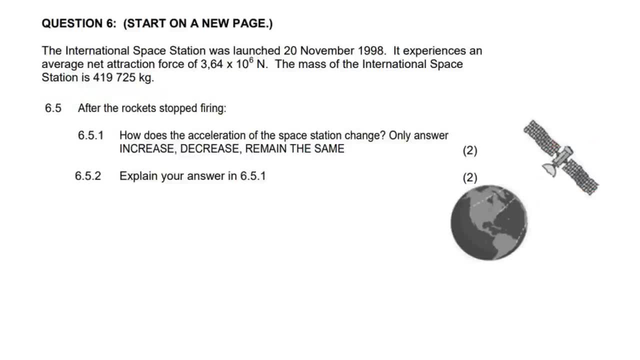 So you can just say that that direction would be away from Earth. OK, Now It is after the rocket stops firing. OK, So what happens was they switched on the rocket and it causes this thing to go at in a certain acceleration. 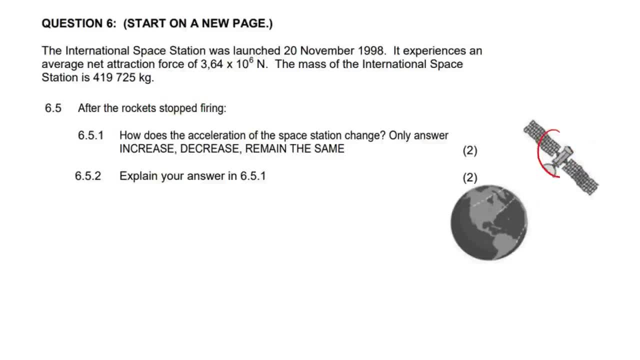 Then they switch the rocket off. OK, But obviously the obviously this would keep going. Right, It's got. it's got a bit of momentum, Newton's first law, things like that. So it says: after the rocket stops firing, how does the acceleration of the space station change? 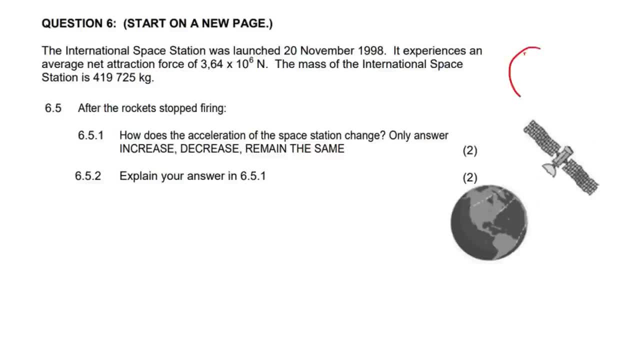 Now think about this carefully. So when the, when the rocket Was accelerating away, the rock- I mean the, the space station- the force of the rocket, with the applied force, would be larger than the gravitational force. That is the only reason that we were able to achieve acceleration. 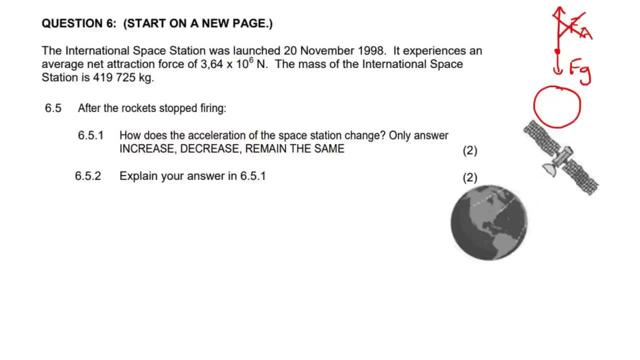 However, when they switch the rocket off, then the only force acting on the object is pulling it back towards Earth. It doesn't mean the rock, It doesn't mean the space station is going to turn around and come back towards Earth, Because it's already gathered a certain speed. 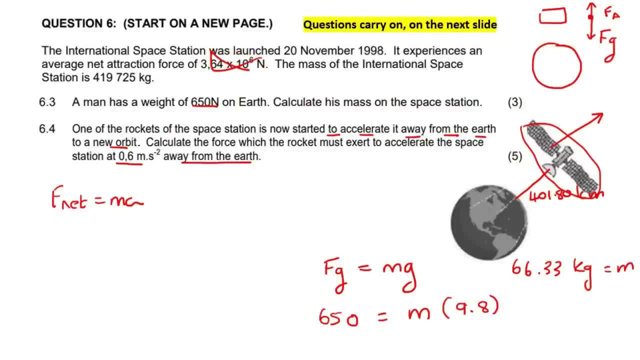 So remember you're fat is not going to be this number anymore. Your F- Steve and Paul- you did a strong influence on the solar system- is going to be the combination of these two. so let's just go say that the f net um will now be: 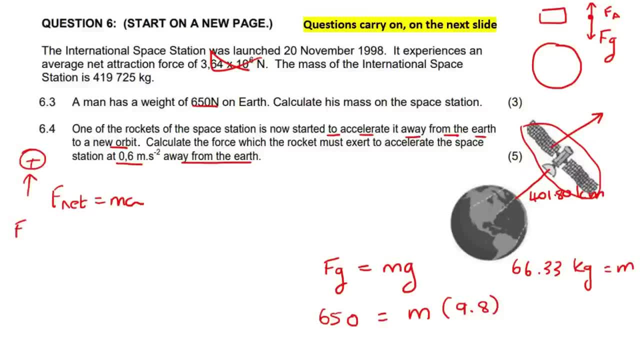 and let's choose going away from the earth as positive. so let's say the applied force of the rocket minus the gravitational acceleration, which is still going to be that at that same distance. right, because as the rocket gets switched on it's still at the same distance. so we can still use. 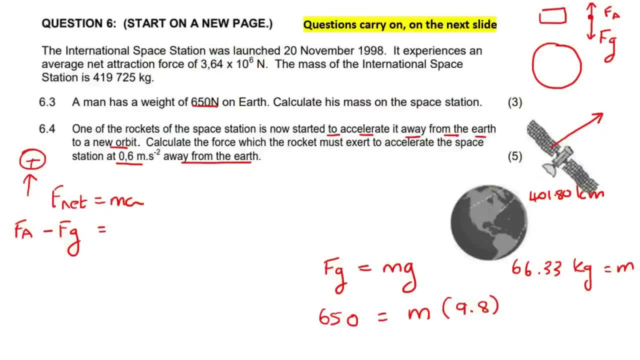 that value, and then we can use the mass of the object. it's always the object, which is 419725, and the acceleration that we are going for is 0.6. so we can then say that the applied force take away 3.64 times 10 to the 6, is equal to all of this. 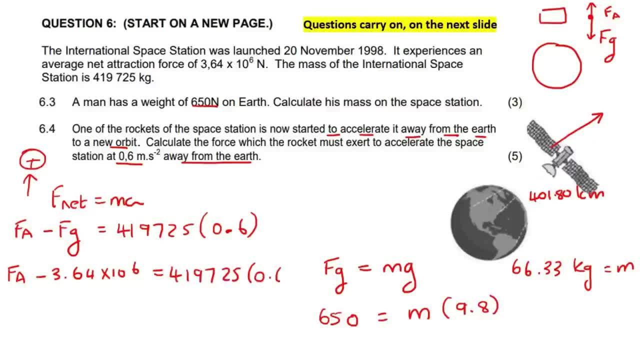 and so if we're to go work out the applied force, we'd end up with 3891835 newtons. so that is the force that one of those rockets would have to exert to cause that 0.6 acceleration. and because it is a force, it's a vector, so you can just say that that direction would be. 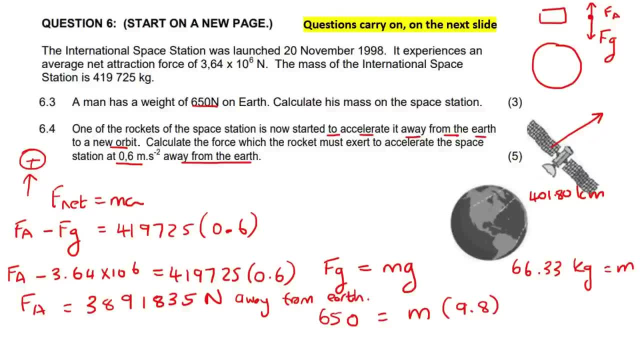 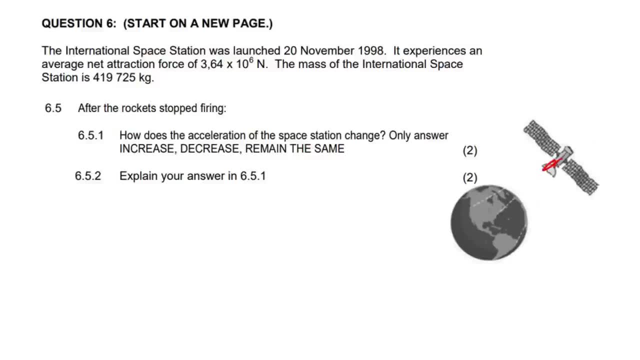 away from earth. okay. now it says after the rocket stops firing: okay, so what happens? was they switched on the rocket and it causes this thing to go at in a certain acceleration. then they switch the rocket off. okay, but obviously, the obviously this would keep going. right, it's got. it's got a. 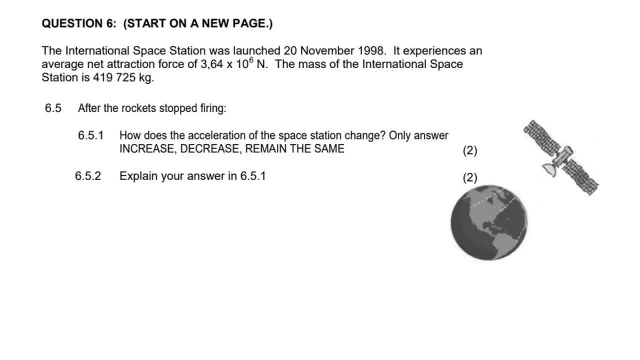 bit of momentum, newton's first law, things like that. so it says: after the rocket stops firing, how does the acceleration of the space station change? now think about this carefully. so when, the, when the rocket was accelerating away, the rock, i mean the, the space station, the. 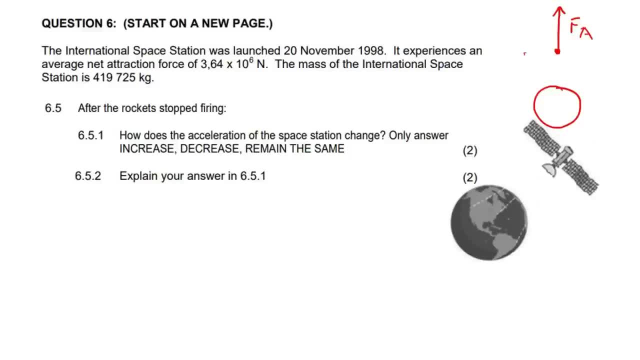 force of the rocket, with the applied force, would be larger than the gravitational force. that is the only reason that we were able to achieve acceleration. however, when they switch the rocket off, then the only force acting on the object is pulling it back towards earth. it doesn't mean the rock, it doesn't mean the space station is going to turn around and